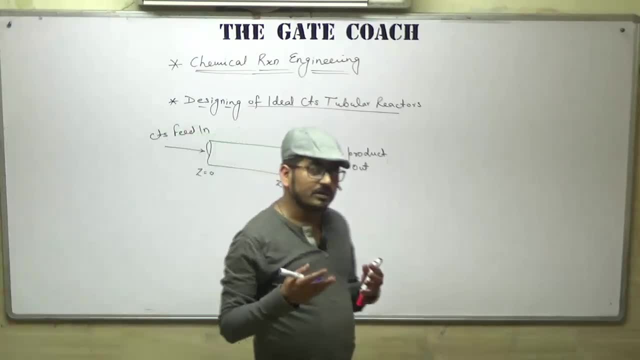 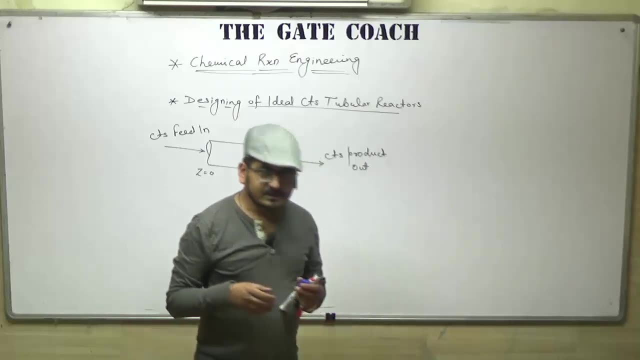 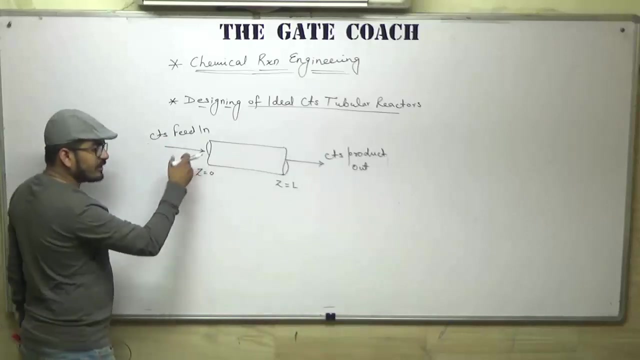 in this reactor, as this is the ideal tubular reactor and we know that the ideal things, the ideal phenomena are imaginary in these worlds. but this is a concept of ideal flow reactor, where the feed is going in the reactor as the ideal flow, and we know that the ideal 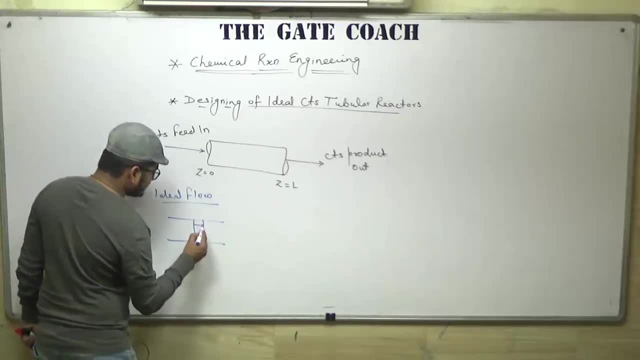 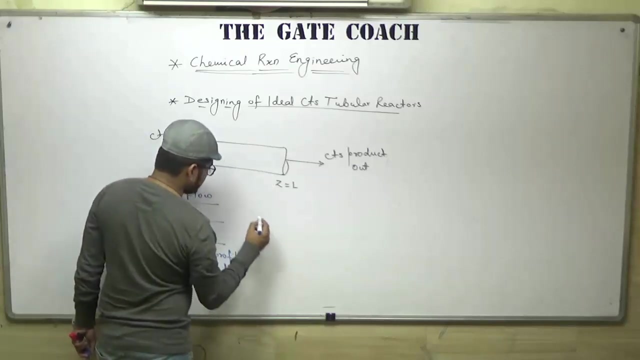 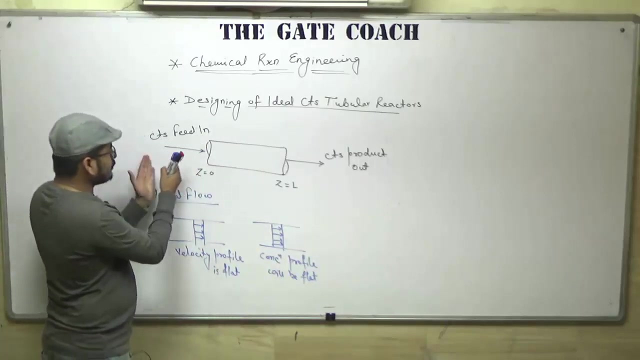 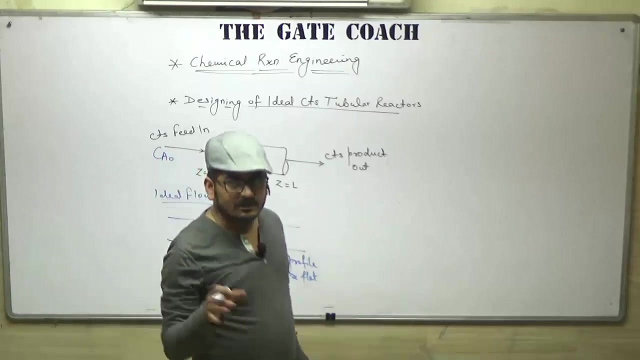 flow is where the viscosity is 0 and the velocity profile is 0. So because of the flat velocity profile, the concentration profile in this reactor will be flat as well. so what is happening in this reactor, like the fluid is going in the reactor and having the initial concentration, let's say CA0, I am assuming that all of you know. 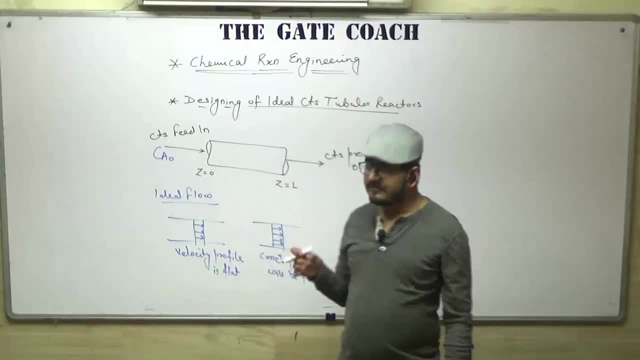 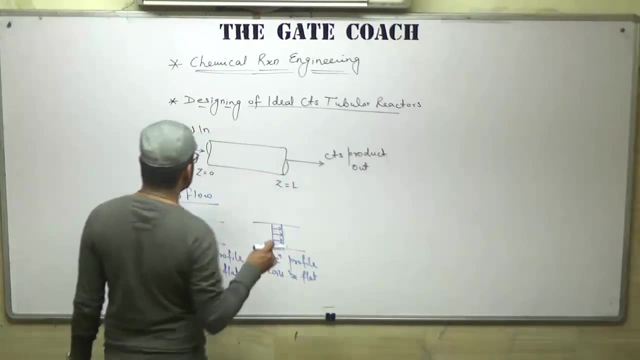 the basic terminologies And the basic meaning of each and every term in this subject. so if you have still any doubt, you can ask that in the comment section. So the initial concentration of any reactant A is, let's say, CA0 that is going in this reactor. 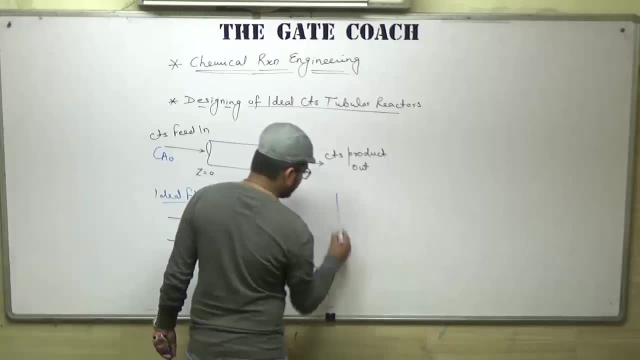 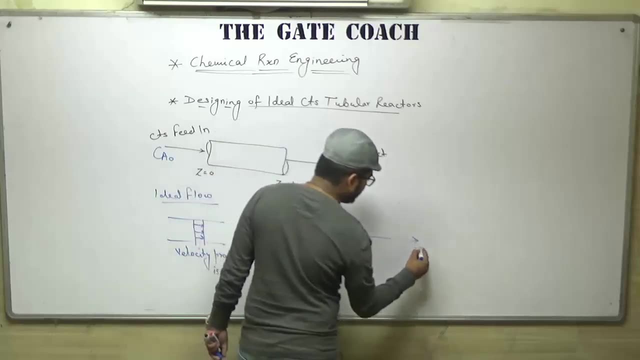 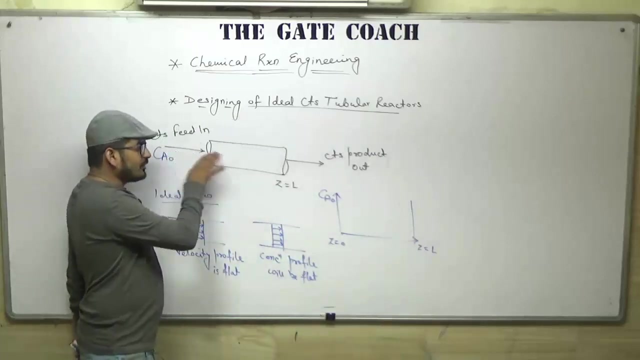 and if we draw the concentration profile for this reactor, let's say like this: at Z equal to 0, the concentration is CA0 and this is Z equal to L. So what happened? CA0 is going in this reactor and as the fluid passes along the length of the reactor, the 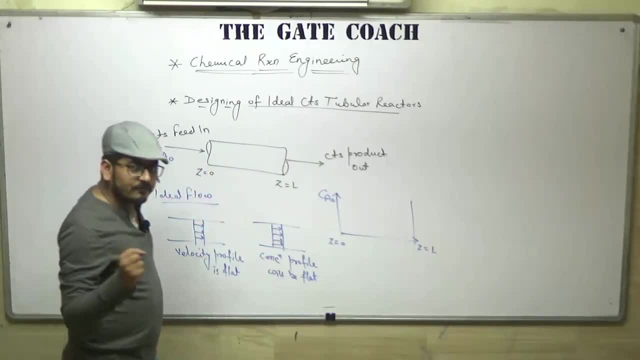 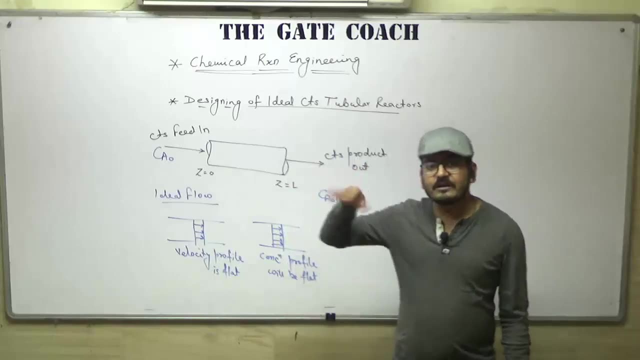 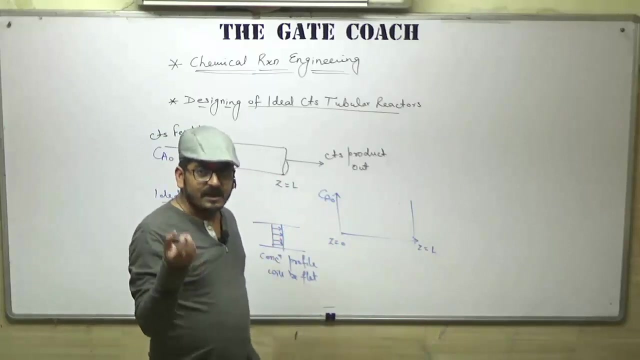 concentration of the A will decrease, because all of us know that the reactant get disappeared in the reactor, the reaction takes place and the A will convert into the product. so that is why number of moles of A present in the mixture will get decreased, and as the number 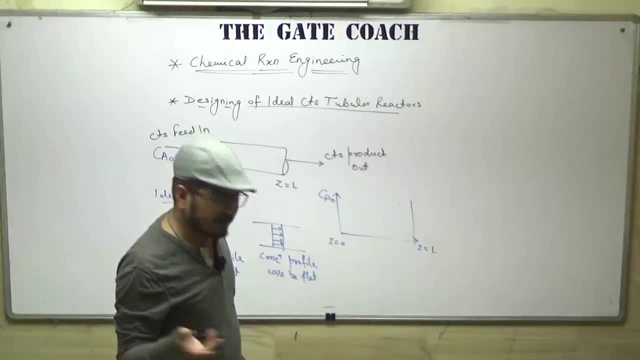 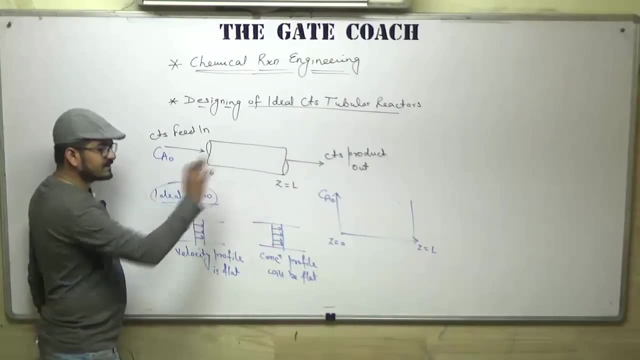 of moles of A are decreasing, The concentration of A will decrease, so the profile will be flat. because the velocity profile is flat, we are assuming the ideal flow in this and that is the basic concept of ideal plug flow reactor. So because of the ideal flow, molecules are moving, all molecules are moving in with same. 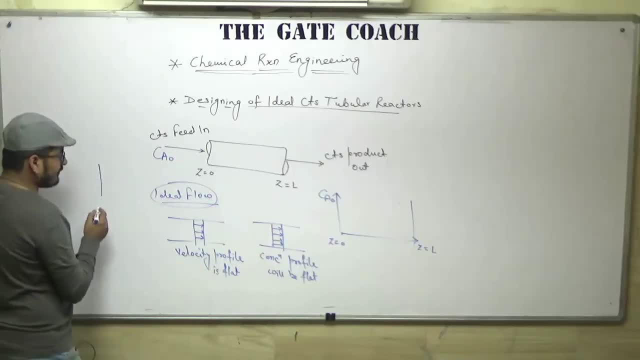 direction means like this: this is the profile. this is the molecule: CA0 concentration at Z equal to 0. So enters in the reactor and as they move, let's say at Z equal to Z1, at another point the concentration of these molecules will decrease, but as we see through the vertical. 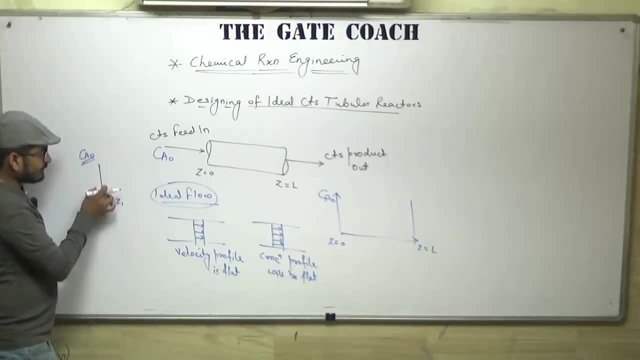 line in this vertical direction. all molecules are moving with same velocity because the velocity profile is flat, so these molecules will move like this, and at this point as well. okay, The concentration will be flat, but less than the initial concentration. here it was CA0 and 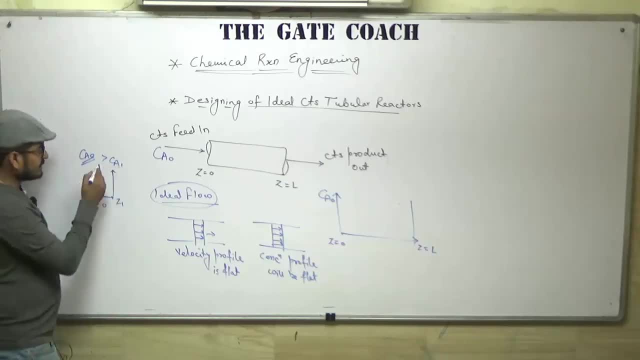 here it will be CA1, let's say, Concentration will decrease but the profile will remain flat, because in vertical direction all molecules are moving with same speed in axial direction, so there will not be any dispersion of the molecule. Okay, And that's why there will not be any dispersion. 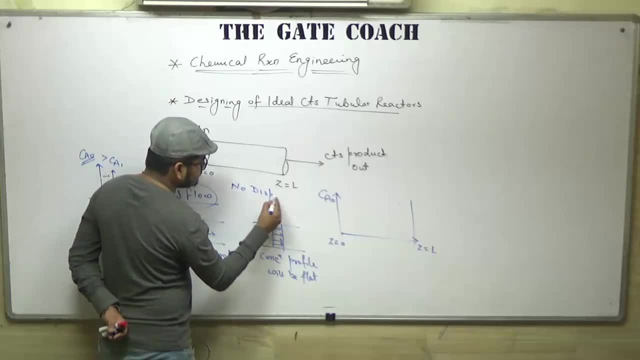 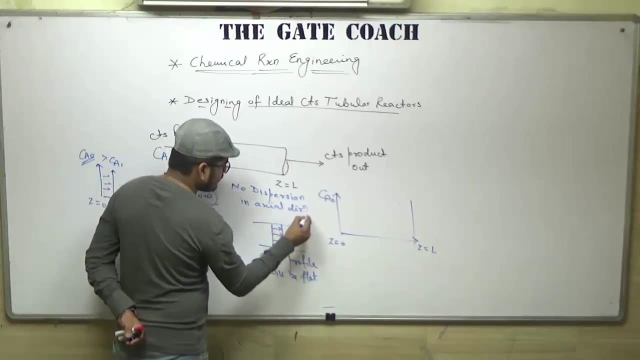 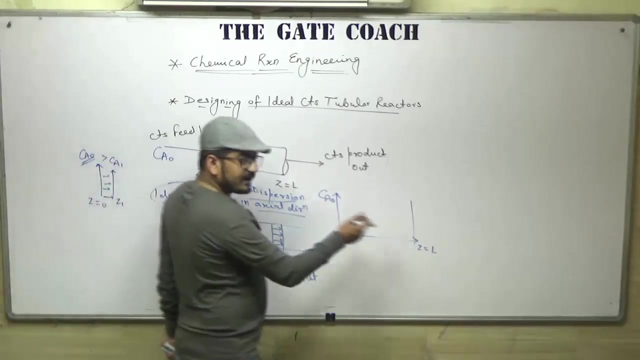 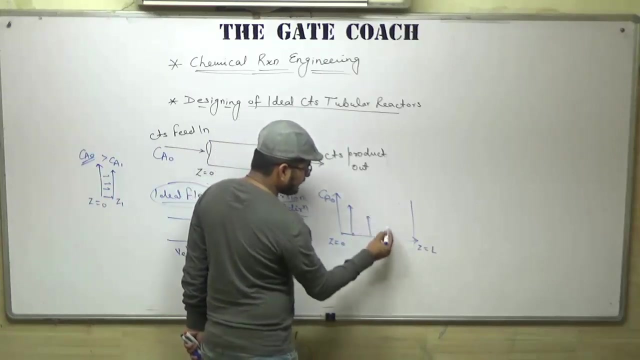 Okay, There will be no dispersion in axial direction. okay, I think we are clear with this. and the profile will be like: CA0 at Z equal to 1, it will be like this: this, this, this: this Profile will be flat. 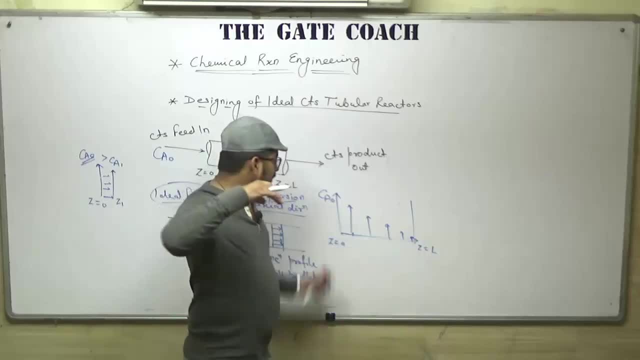 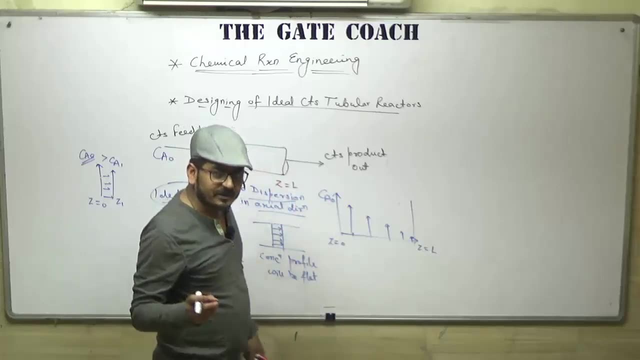 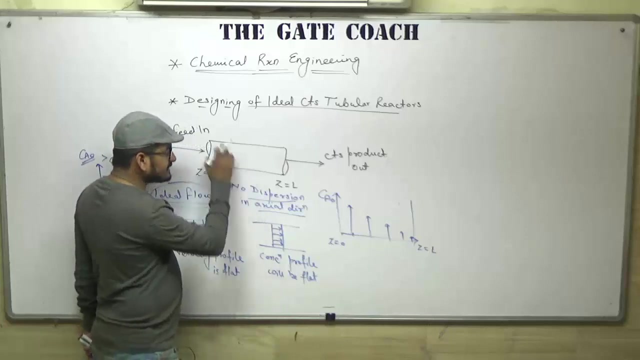 Okay, But the magnitude of this concentration will decrease because along the length of the reactor the concentration will decrease. for reactant A it will convert into product, Okay. So I think it is clear to all of you why we say in these type of reactors, all molecules. 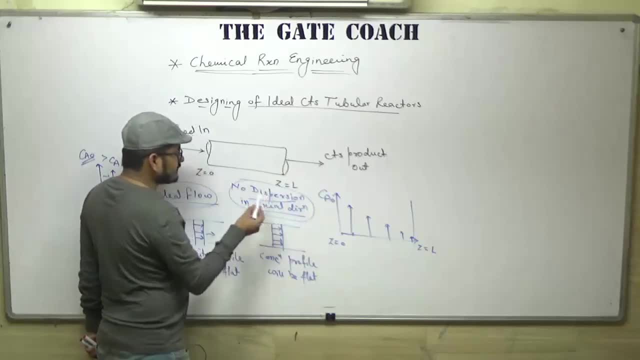 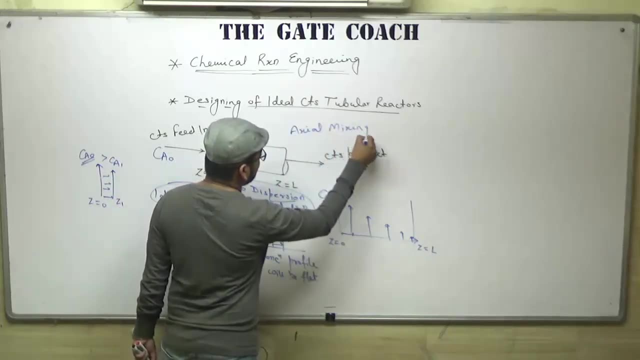 are moving with same speed, then the dispersion in axial direction is 0, so we can also say: when there is no dispersion, Okay, When there is no dispersion between the molecules in axial direction, so the axial mixing will be 0. Okay. 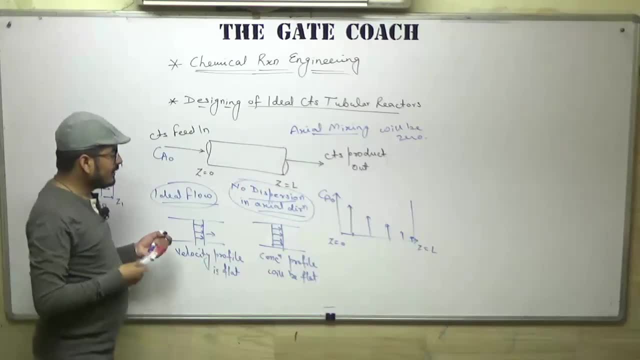 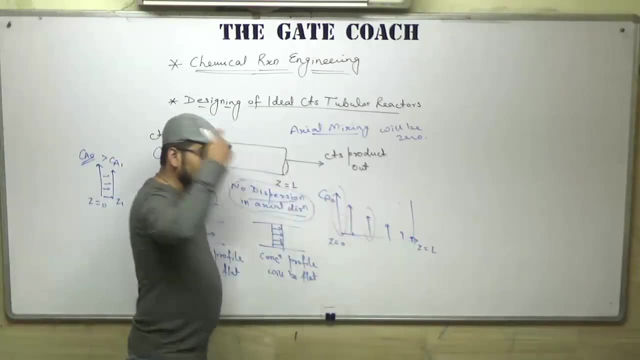 But in vertical direction. we can see in vertical direction that throughout the reactor, throughout that line, concentration is uniform and it is possible only when the mixing is infinite. Okay, We have very high rate of mixing, As all of us know. we have very high rate of mixing. 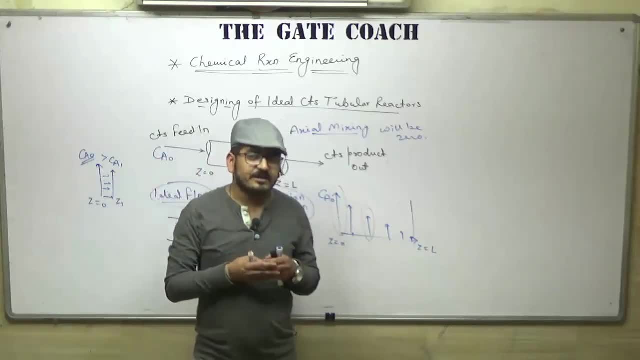 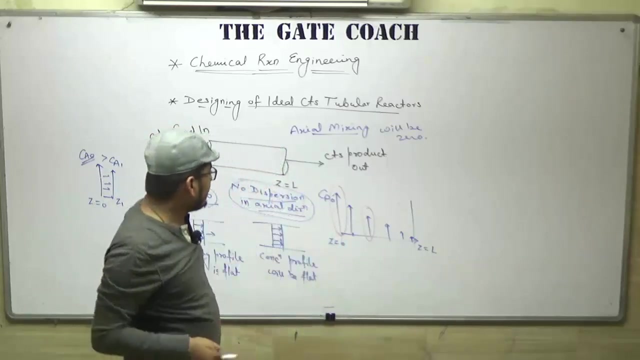 As all of us know that we have discussed batch reactors, we have discussed mixed flow reactors. Okay, So whenever in any mixing tank the rate of agitation, rate of mixing, is high, the concentration distribution in that mixing tank will be uniform, In the same way as we can see in vertical direction, in vertical line concentration. 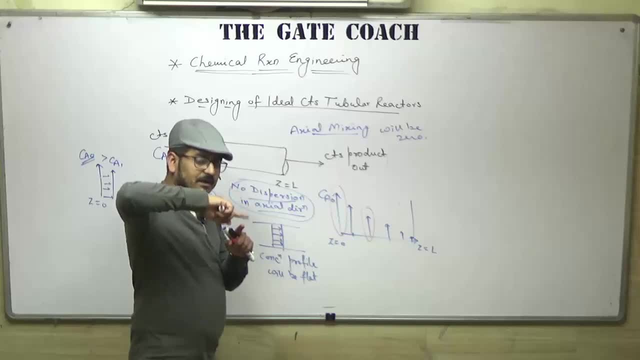 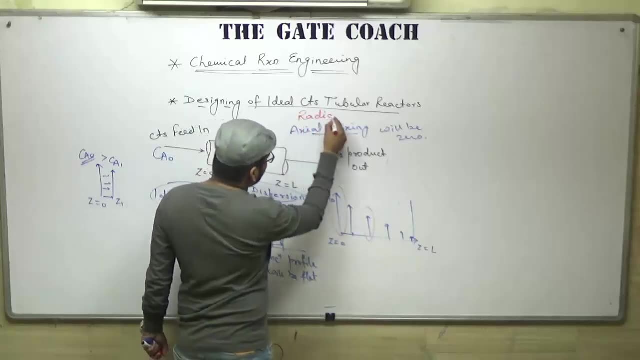 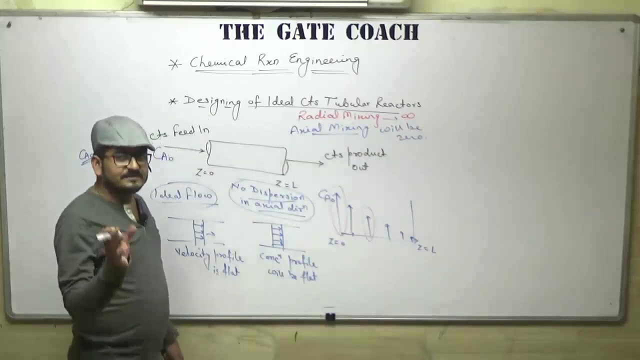 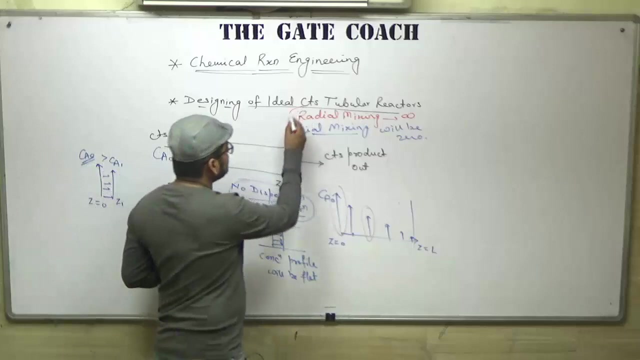 is uniform. it simply means must be there is some mixing. Okay, So we can see that. we can say that in radial direction the mixing is high, or radial mixing is infinite. Okay, That is one of the important characteristic of ideal tubular reactors, as we can see that. 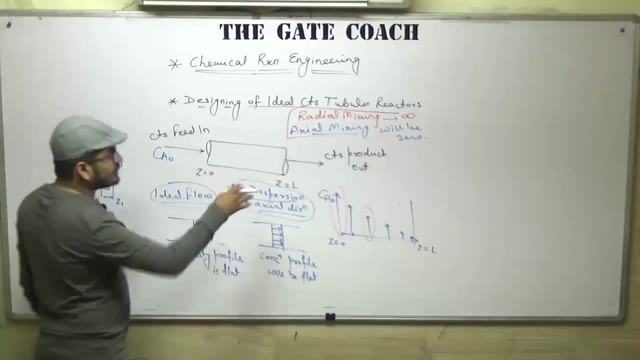 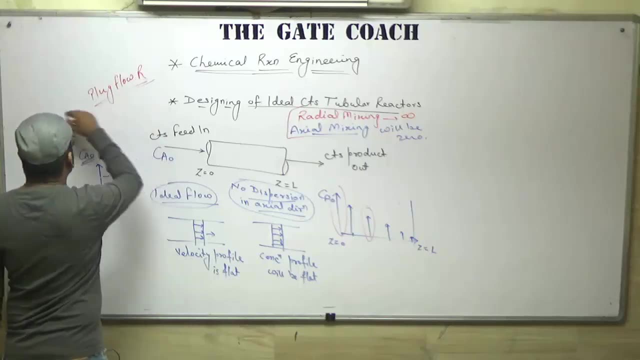 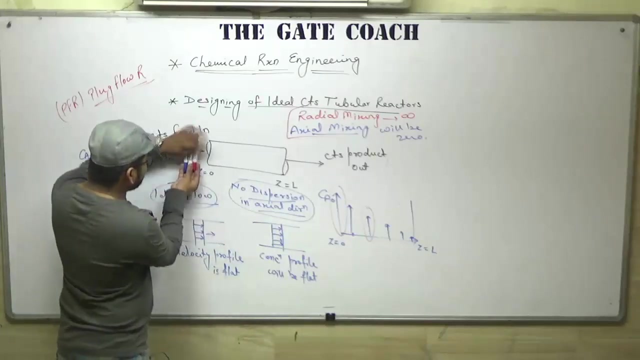 Okay, Now the second point, this ideal tubular reactor, also known as plug flow reactor, Or you can say PFR, Why? Because of the ideal velocity profile, all molecules are moving with same speed and we can say, since all molecules, like you can see, these are the three layers, feed is going. 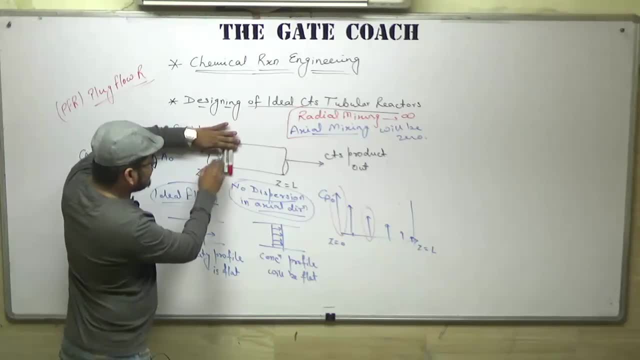 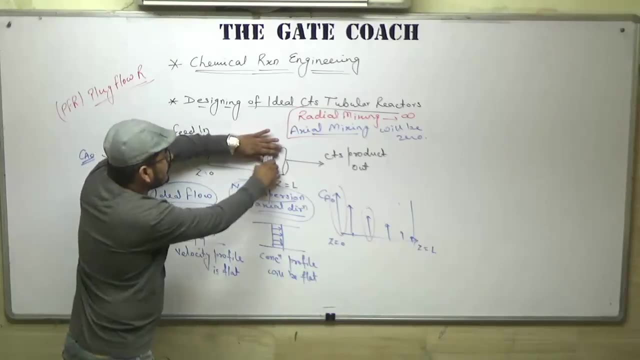 in the reactor, all molecules are moving with same speed and their respective concentration is decreasing, But there is no interaction between these molecules. Okay, So we can see all fluid particles are moving in a plug, in a line, in a vertical line. 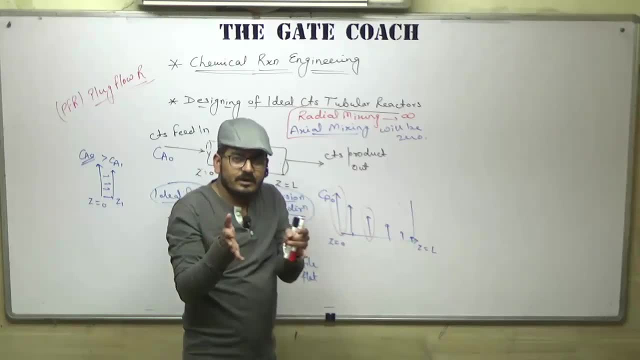 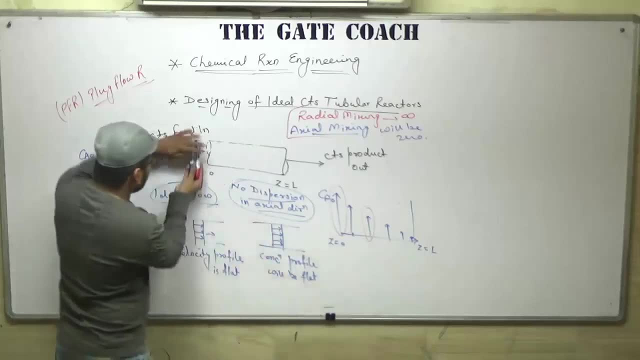 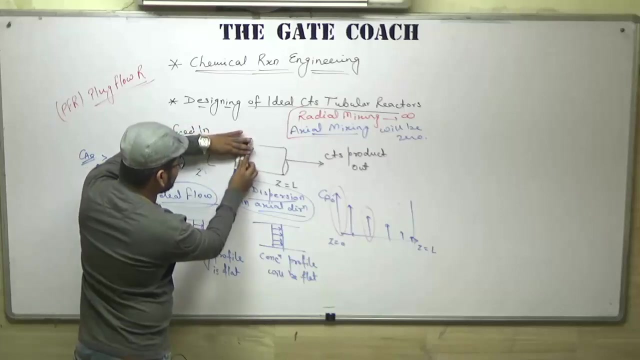 and those vertical lines are different. Okay, So means those vertical lines are like plugs, So all fluid particles are moving in the form of plug. One plug is moving, another plug is moving and the third plug is moving behind that, But there is no interaction because axial mixing is zero. 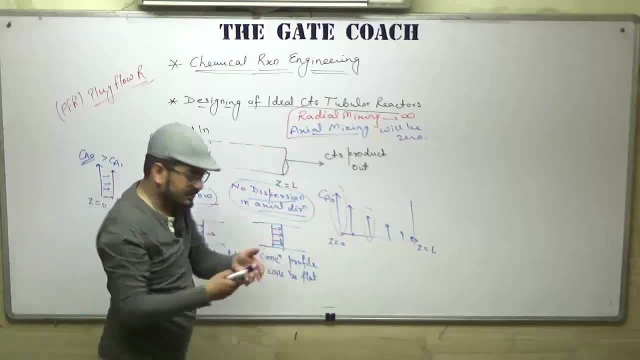 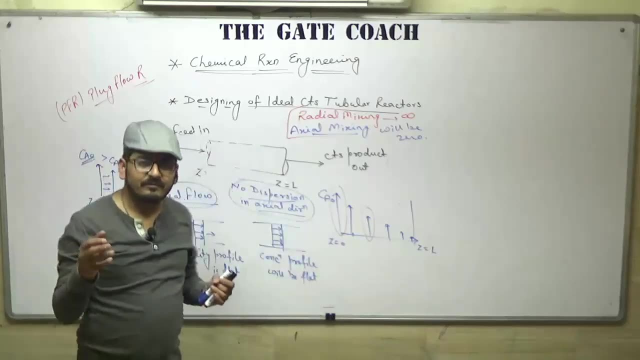 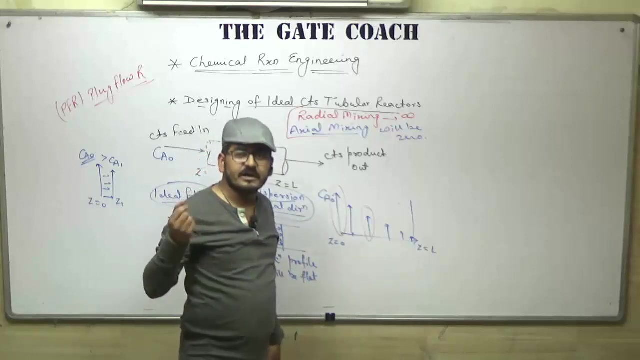 So we can see, Fluid is moving in the form of plugs. That is why it is known as plug flow reactor. If you want to relate it, you can relate it by the daily life example. Let us say, when we go in any queue, in the queue of movie tickets or flight tickets, or 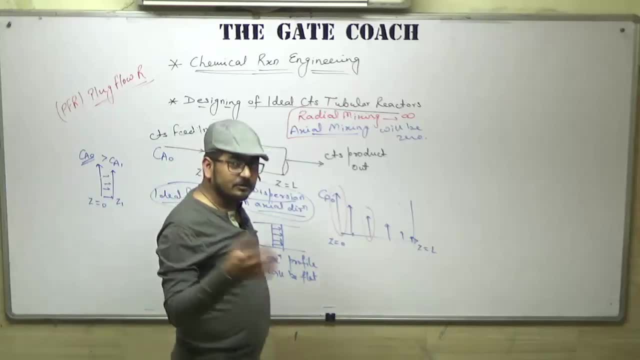 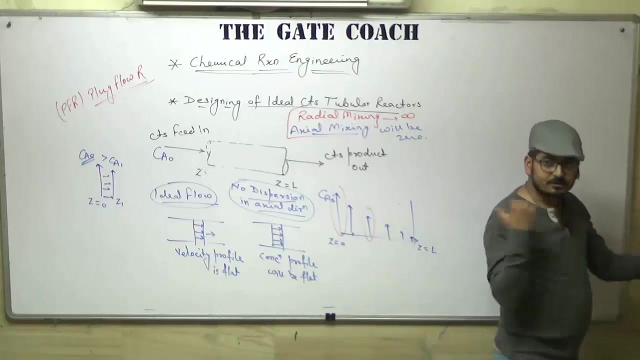 railway tickets in the queue. we are there and normally we do not know who is the person in front of us and in back, in back side us. So what happened? We move like this and there is no interaction with that person next to us. 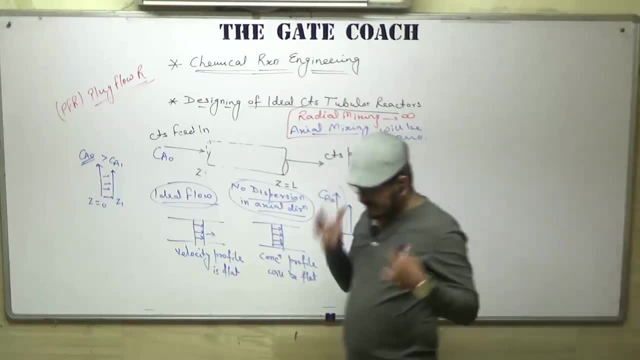 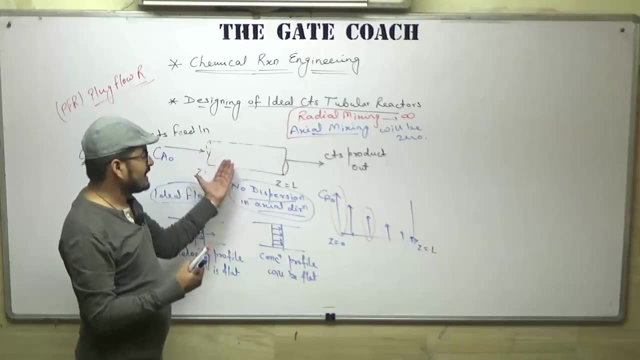 Okay, And we collect the ticket and move on. So, as an individual, we are moving. So, in the same way, fluid particles move as an individual layer, as individual plug in this length and when their work happened, the all process happened, they leave the reactor. 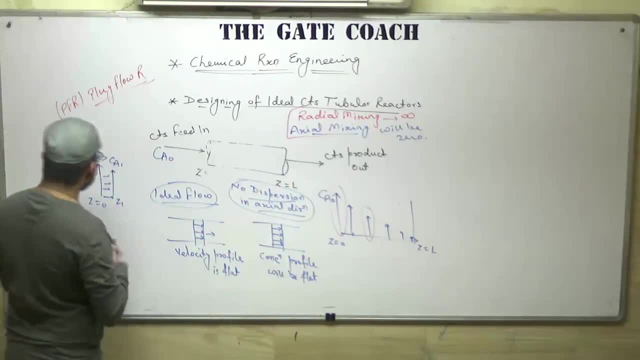 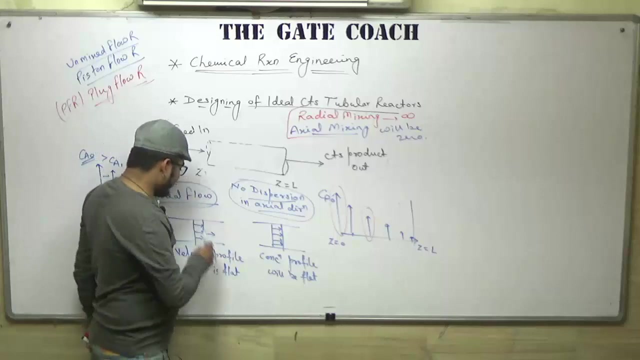 Okay, So this is plug flow reactor And in the same way, it is also known as piston flow reactor and unmixed flow reactor. Unmixed because in actual direction mixing is zero, and piston flow because, you can see, the velocity profile is flat, just like the cylinder and piston assembly. 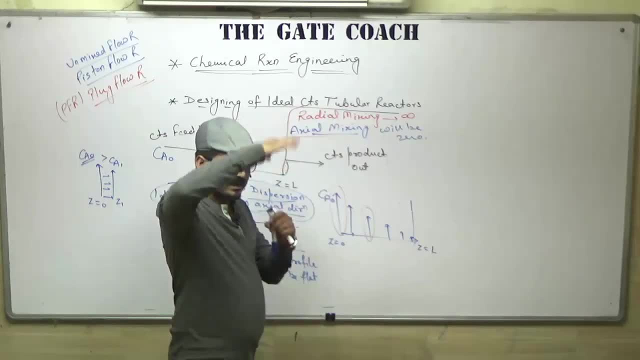 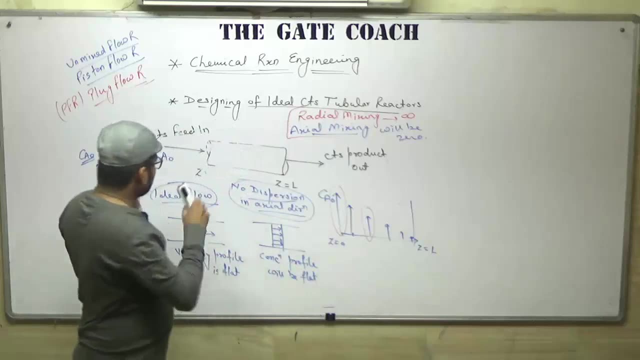 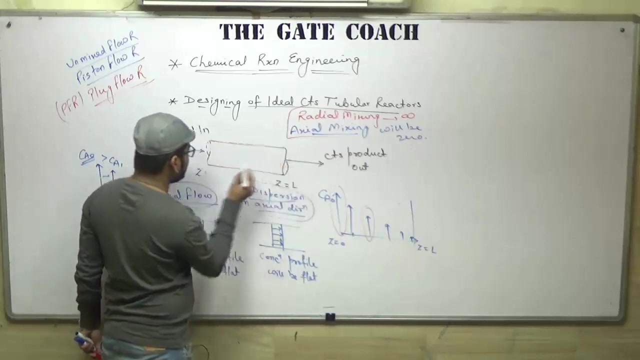 In cylinder and piston assembly. piston moves like this: Okay, The all gases feel the same pressure, in a flat direction. Okay, So that is why, So this is clear to all of you. And one important thing I would like to say in this plug: flow reactor, as we can see along. 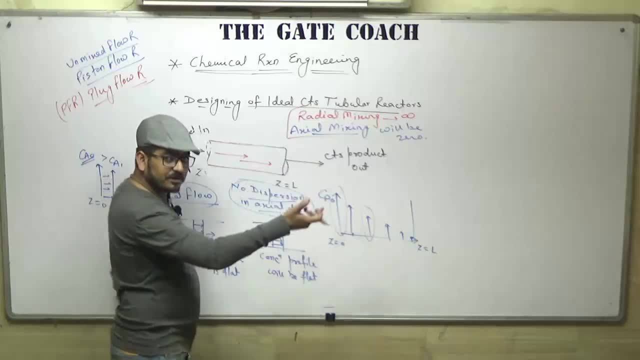 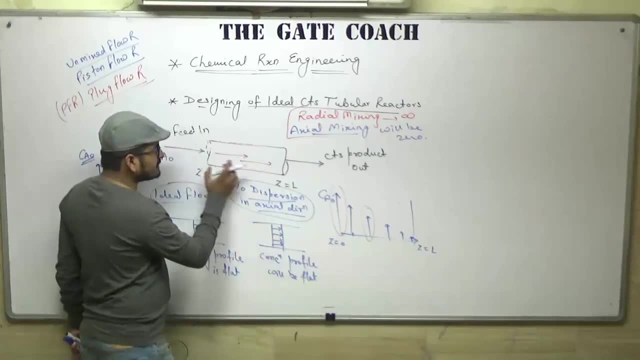 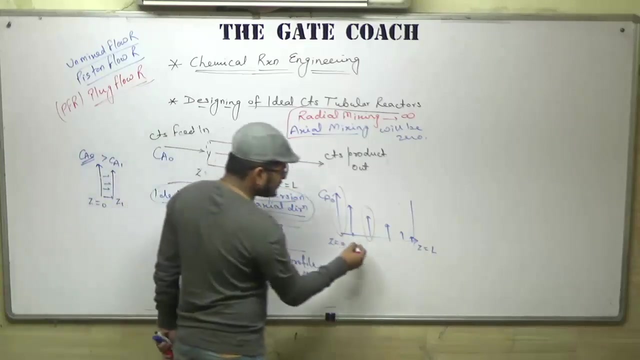 the length of the reactor concentration is changing because molecules are reacting and converting into product. Okay, So along the length concentration is changing. So we can also say As At different points we have different concentration. we can see in this profile. 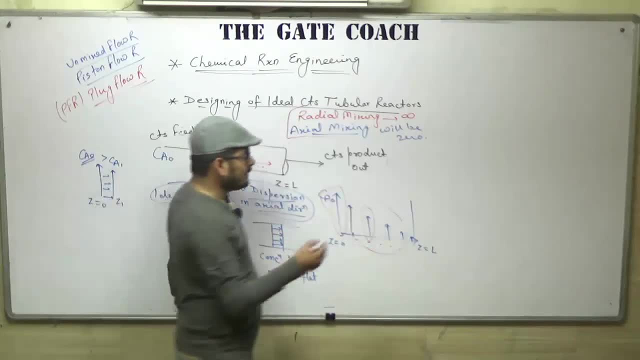 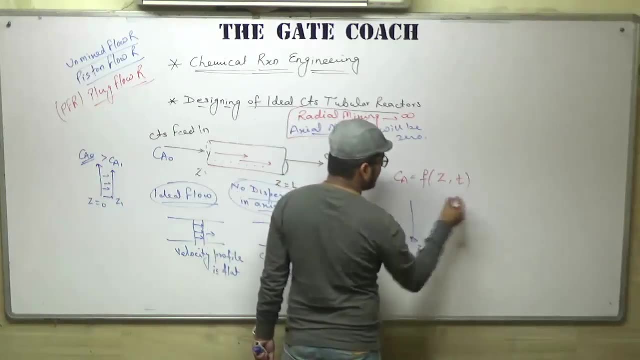 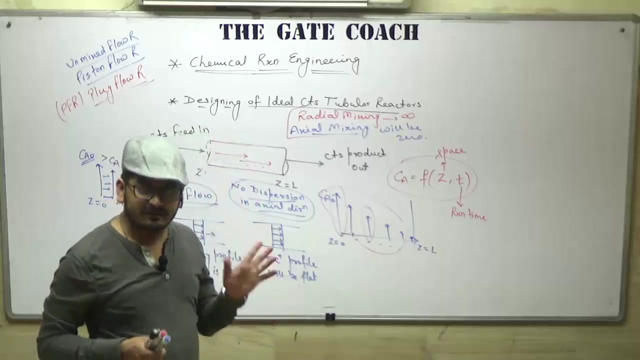 At different points we have different concentration. So we can say that here concentration is the function of length as well as reaction time. Length or you can say space. Okay, So these are two main characteristics of plug flow reactor. I am repeating once again. 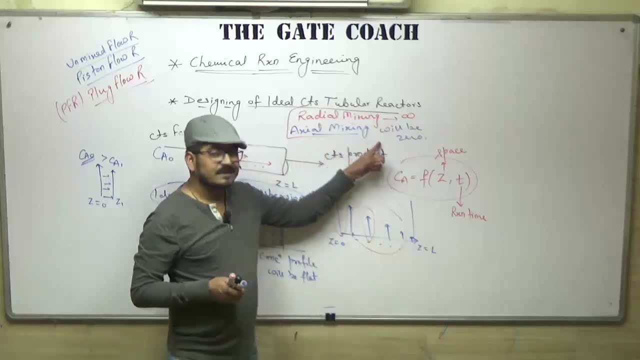 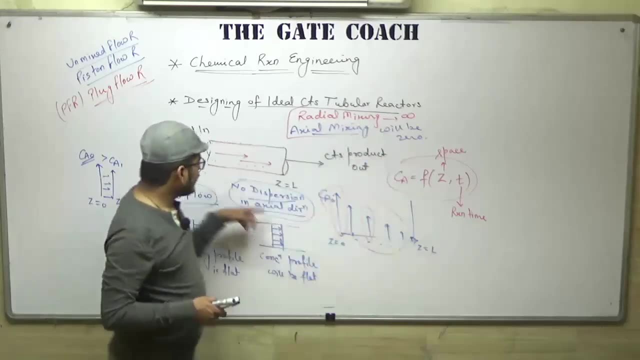 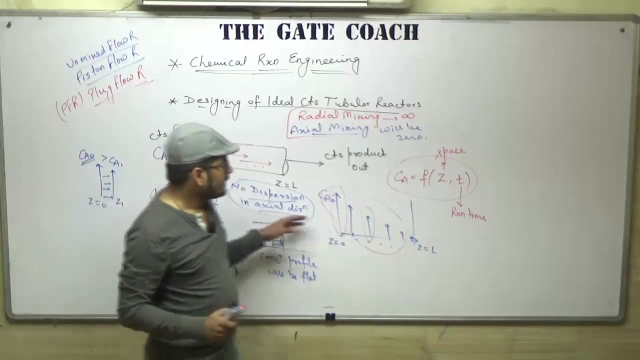 First, the actual mixing is 0 because of the flat velocity and flat concentration profile, And radial mixing is infinite because in vertical direction concentration is uniform and that is possible only because of the high rate of mixing, Okay. And second, as the length, along the length of the reactor, concentration changes. 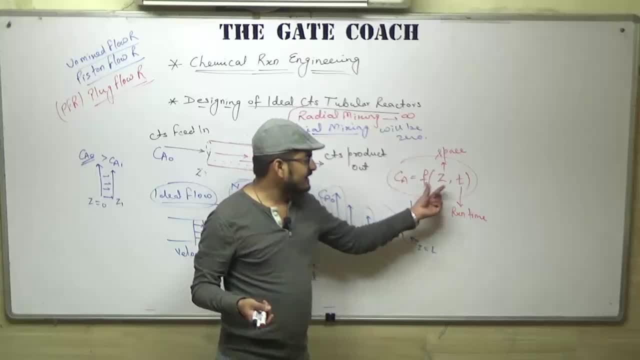 So concentration is a function of length as well as reaction time. Okay, So this is something about plug flow reactor. Now we will talk about the design equation of plug flow reactor. Okay, So now let us draw a PFR. 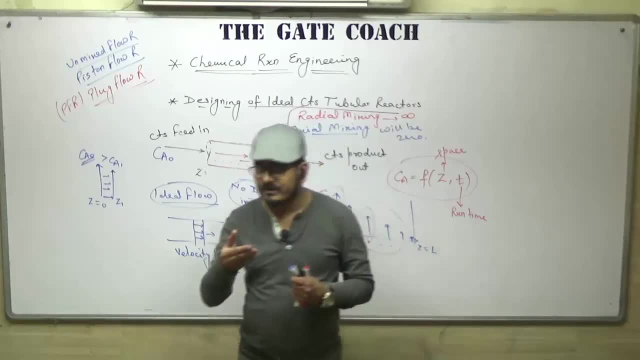 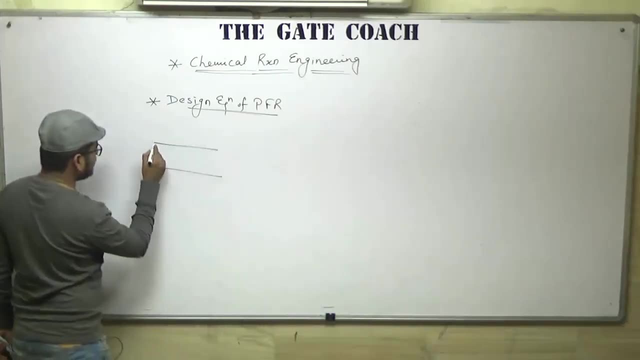 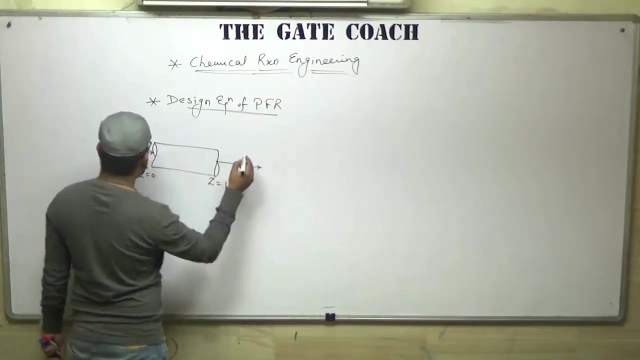 Length is Z equal to 0 to Z equal to L, The feed is going in, The flow rate is V, naught Volumetric flow rate is V0 and the concentration, let us say CA0. and at outlet volumetric flow rate is V0. let us say why: because all continuous flow reactors operates at steady state condition. 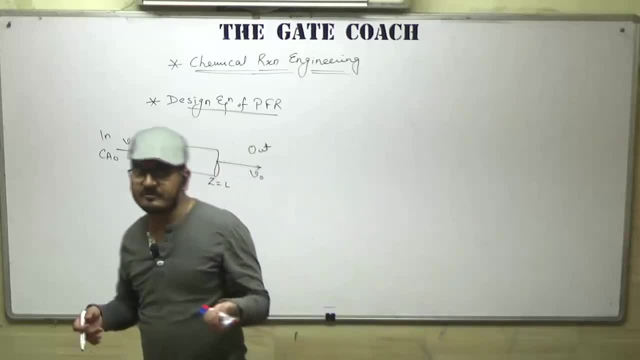 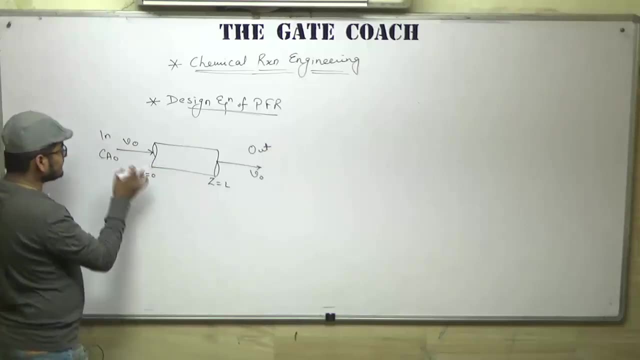 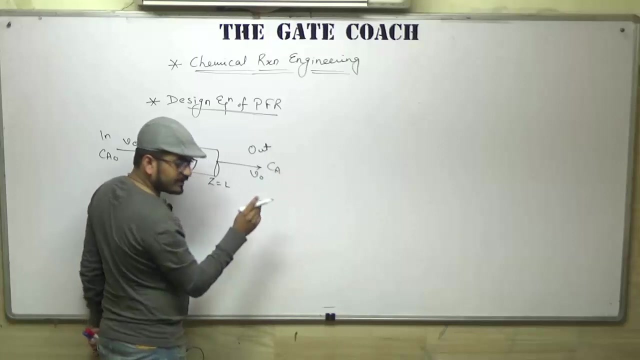 all of us know that we have discussed that in the time of designing of MFR. So all flow reactors operates at steady state condition. that is why the volumetric flow rate at inlet and at outlet will be same and the concentration is, let us say, CA, the final. 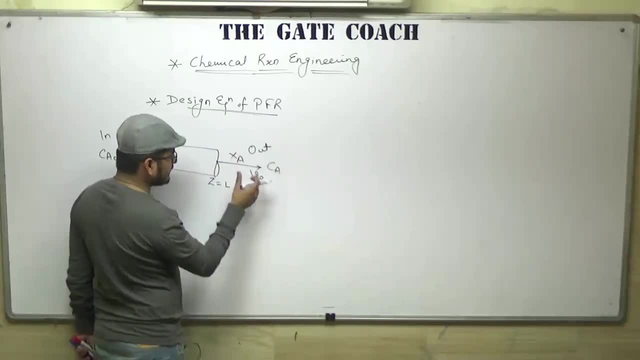 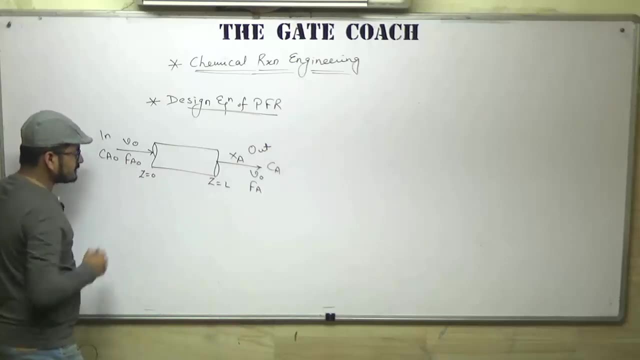 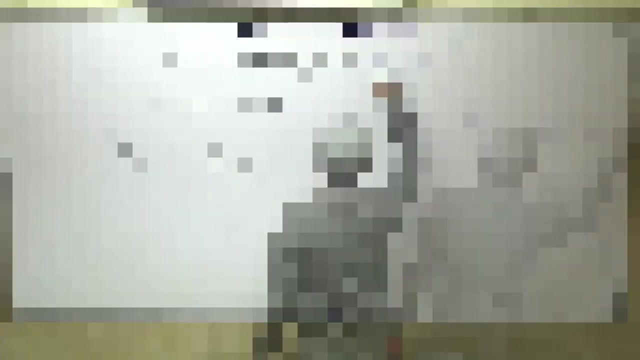 concentration desired conversion XA we have achieved at the outlet and the molar flow rate of A at the outlet is FA and at inlet let us say that is FA0, and from the general mole balance equation we know that. so from general mole balance equation we know that. 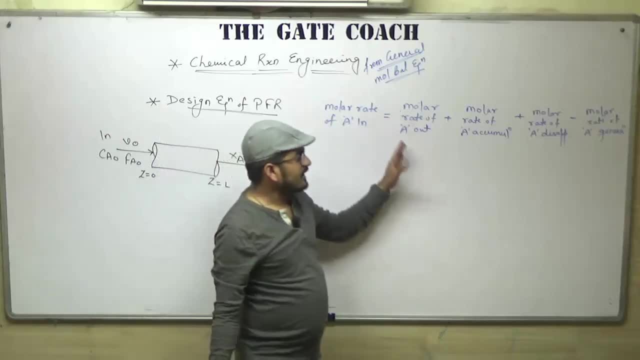 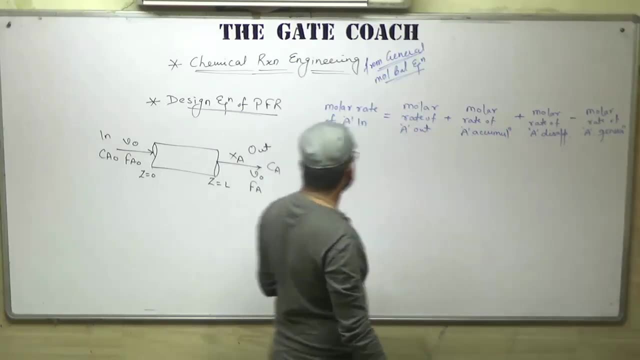 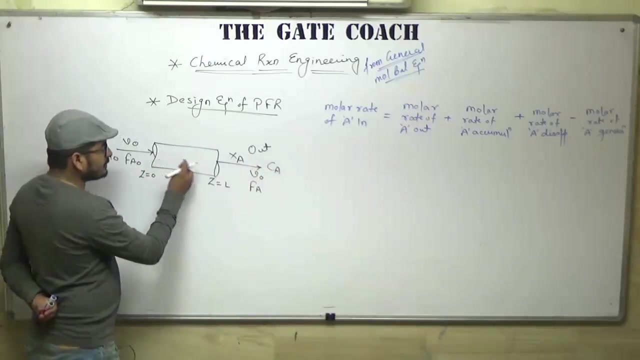 molar rate is V0. So the molar rate of A in will be equal to molar rate of A out, plus molar rate of A accumulation, plus molar rate of A disappearance, minus molar rate of A generation. So in this case, if you see, as we have discussed earlier, that along the length of the reactor 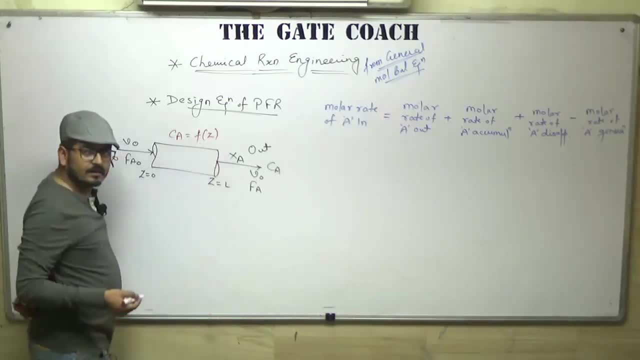 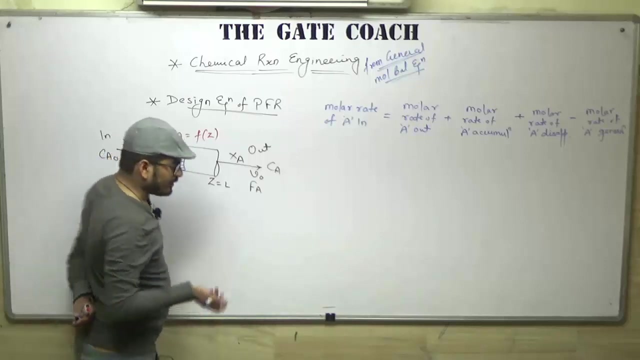 concentration is changing. so it means we cannot apply mole balance for entire reactor. so in that case what we will do, We will take a differential strip and we will do material balance across that strip and then we will integrate. we will do material balance in differential form. so let us say the thickness. 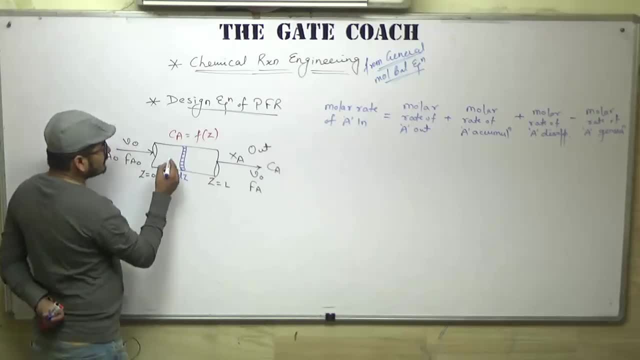 of this strip is DZ, the molar flow rate of A going in this FA and molar flow rate of A leaving this strip is FA plus DFA. So we will integrate, So we will integrate, So we will integrate. DFA is the molar flow rate. 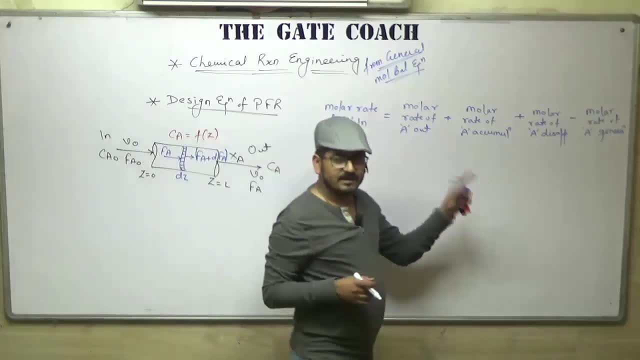 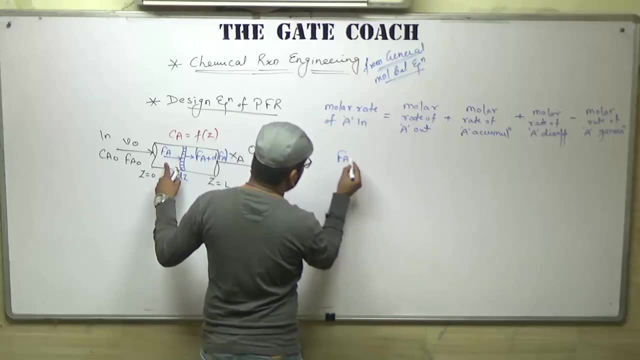 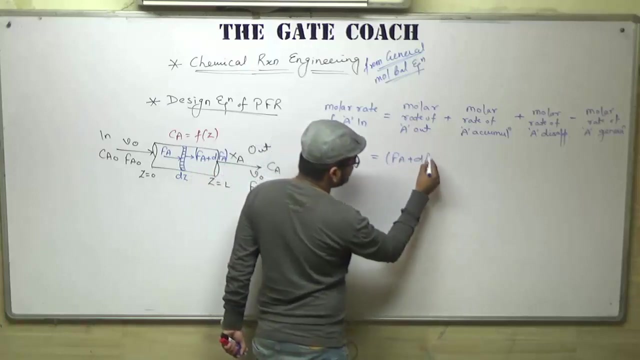 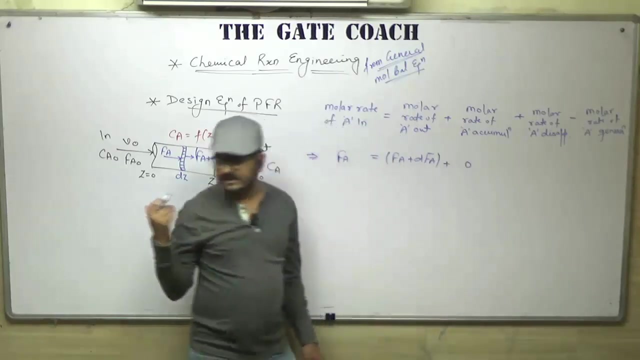 So along the differential strip, when we do material balance and we put all the values in this equation, it will be like molar rate of A in, as we can see FA, moler rate of A out, FA plus DFA, Molar rate of A accumulation will be 0, because this reactor is operating at steady state. 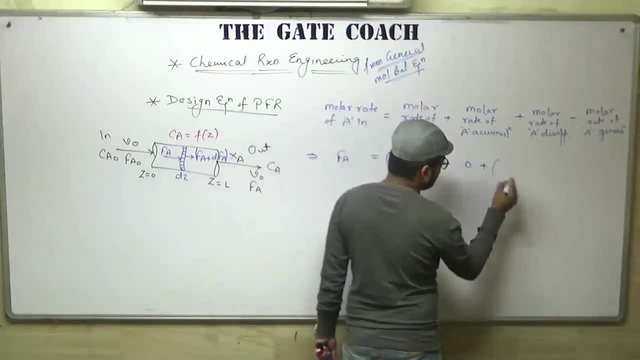 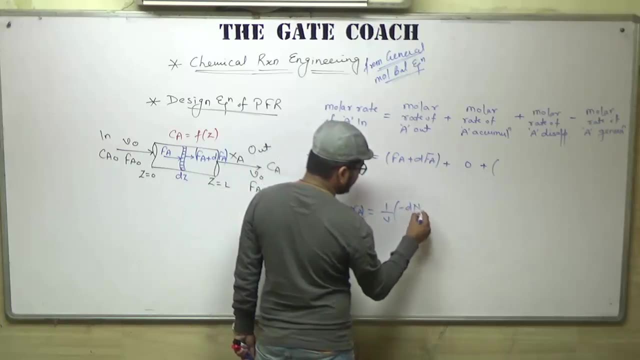 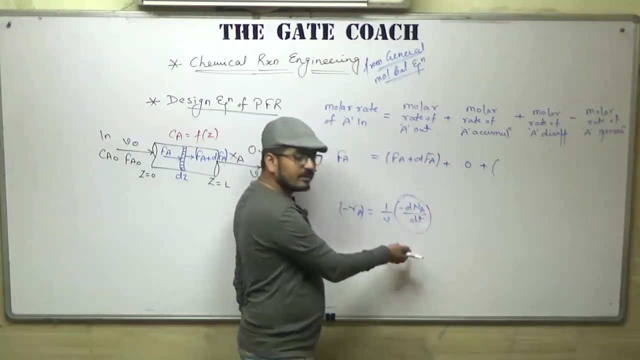 condition: molar rate of A disappearance. we know that rate of reaction defined as 1 over V, minus DNA by DT for any reactant. So here this DNA over DT means minus DNA over DT, is the molar rate of disappearance of A change in moles of A per unit time. So if we write, 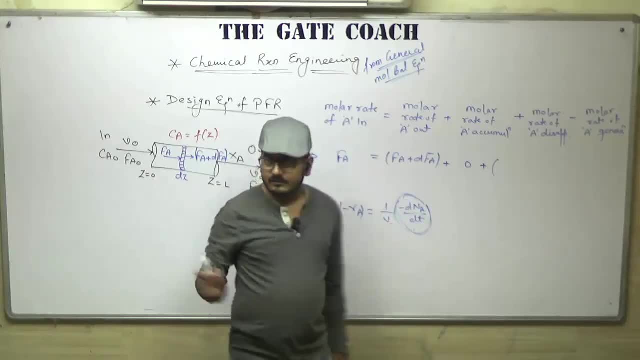 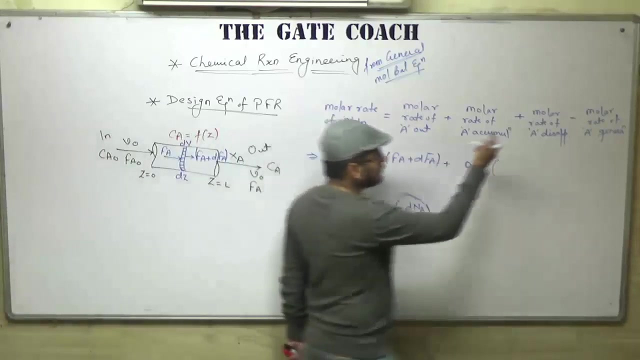 it will be like RA into V, but we are doing this for differential strip and this V is the volume of reaction mixture. So in this strip the volume of reaction mixture will be DV. So the molar rate of A disappearance will become minus RA into DV and generation. 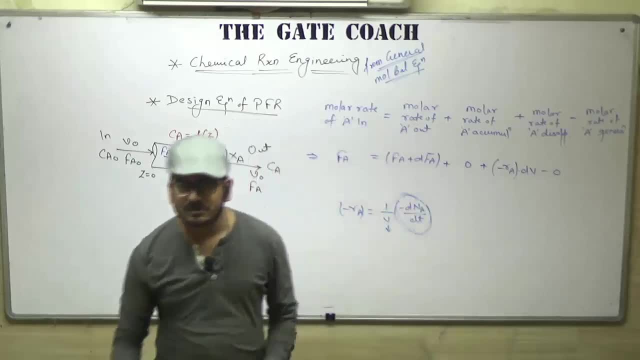 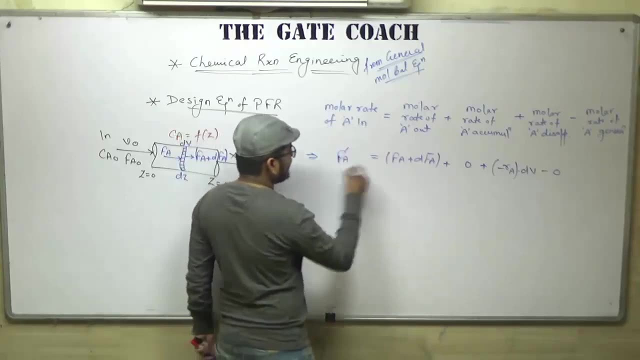 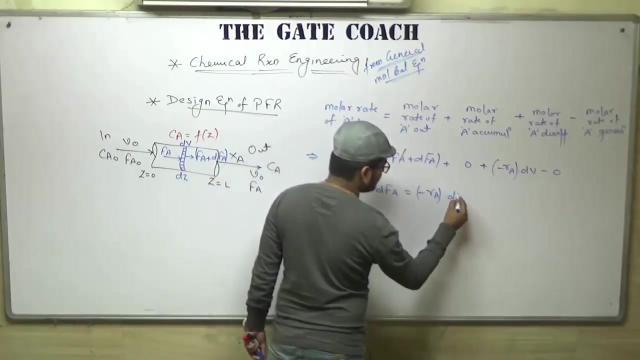 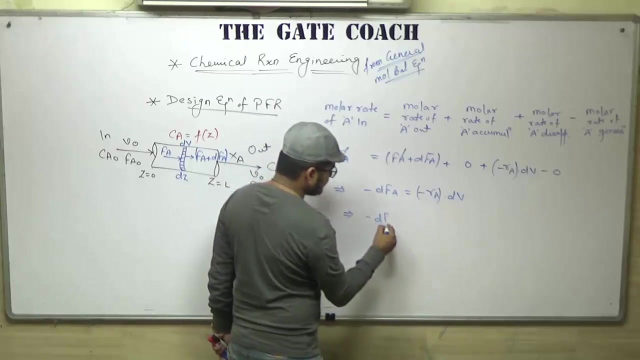 will be 0, because A is the reactant and it will not generate, it will disappear only. Okay. So FA and FA will get cancelled and it will be like minus DFA is equal to minus RA. Okay, And we know that FA is the molar flow rate, So we can write it as FA naught 1 minus XA. 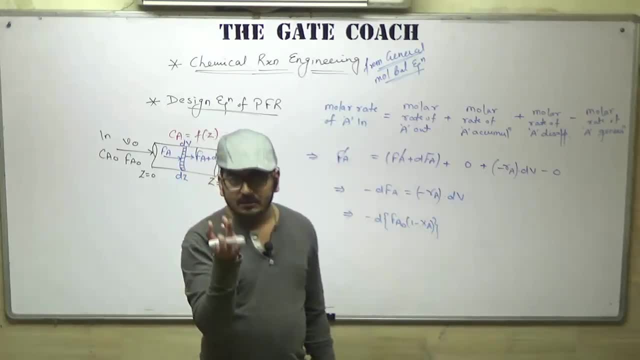 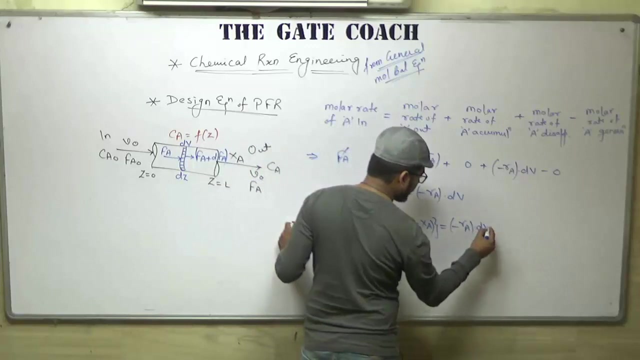 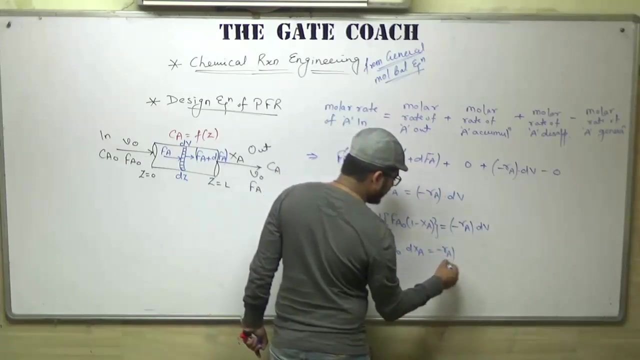 because ultimately, in any reactor, the desired objective is: the desired objective is to achieve the final reaction, The final conversion, the desired conversion. Okay, So we have to write it in terms of conversion and it will become like FA naught into DXA is equal to minus RA into DV, or you. 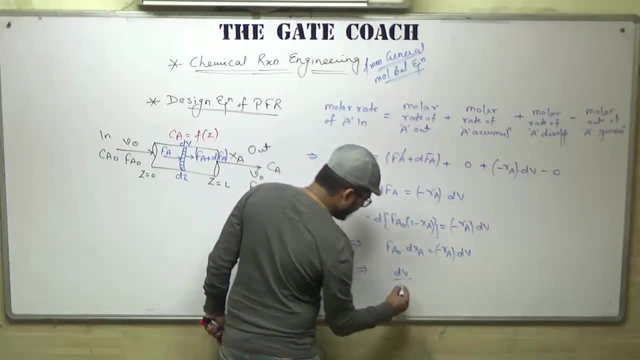 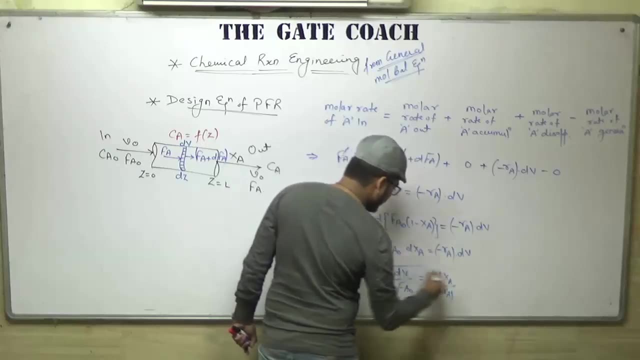 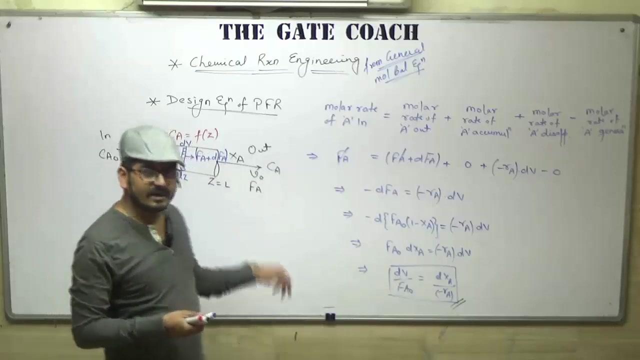 can write it as: DV over FA. naught is equal to DXA over minus RA. Okay, Okay, Okay, Okay. So this is the design equation of ideal PFR in terms of conversion in differential form. Okay, Now, if we talk about the integral form for overall reactor, then we have to integrate: 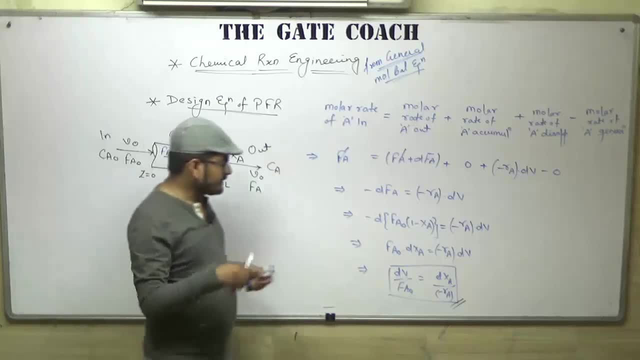 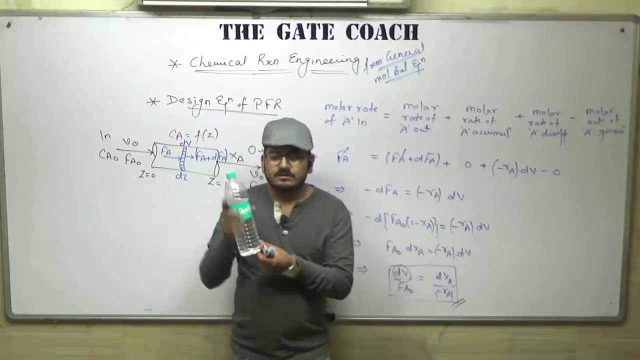 that Okay, But now, before that, I just want to make you clear what is the meaning of this DV. Okay, As all of us know that if we want to store One litre water, then to store one litre water, or one litre of any component, we need the 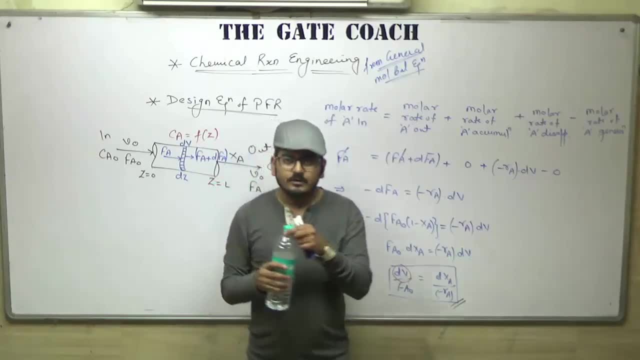 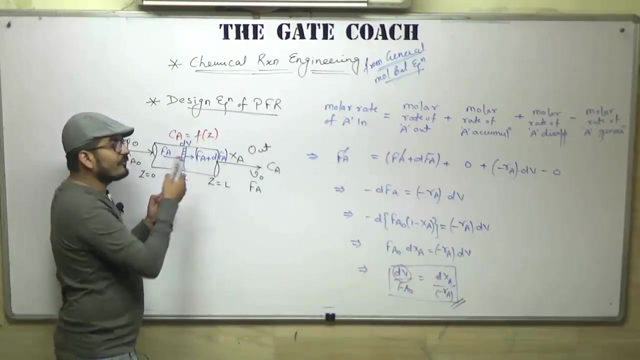 minimum one litre of vessel. Okay, To store one litre of liquid or gas or whatever it is, we need minimum one litre of vessel. In the same way, to store two held DV volume of reaction mixture, we must have one litre of vessel. We must have minimum DV volume of reactor. 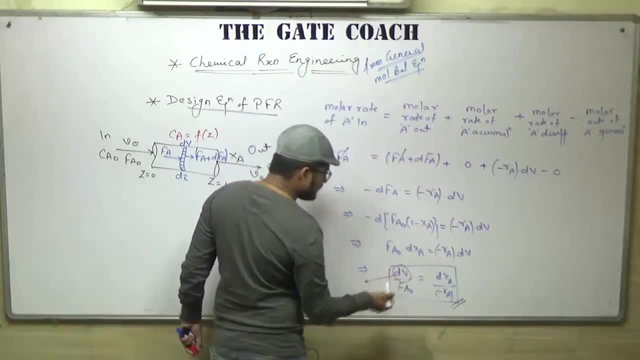 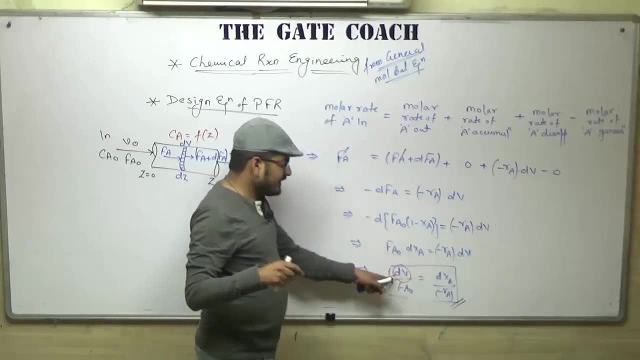 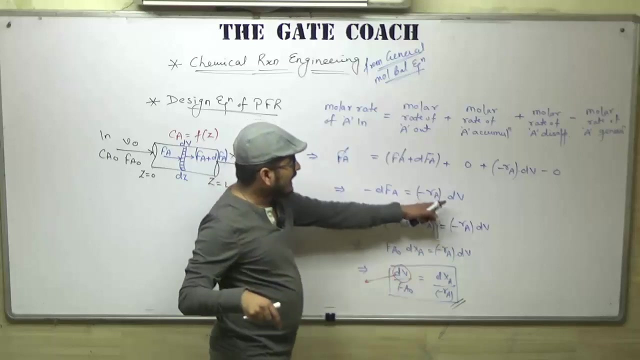 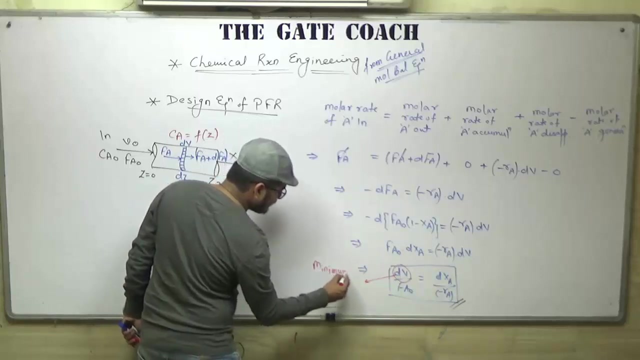 Okay, So this DV, which we said was the volume of reaction mixture in this differential element, Now we can also say: this is the minimum volume of reactor required to held DV: volume of reaction mixture. Okay, Okay, So now let us move on. 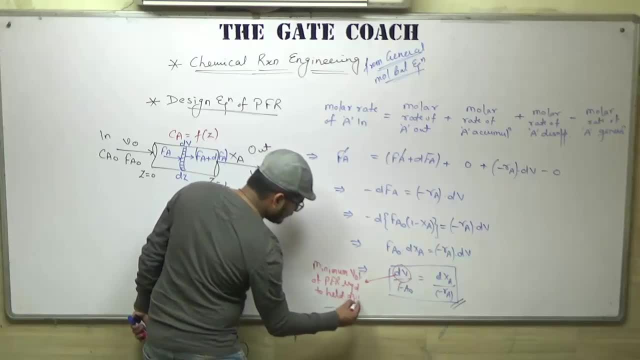 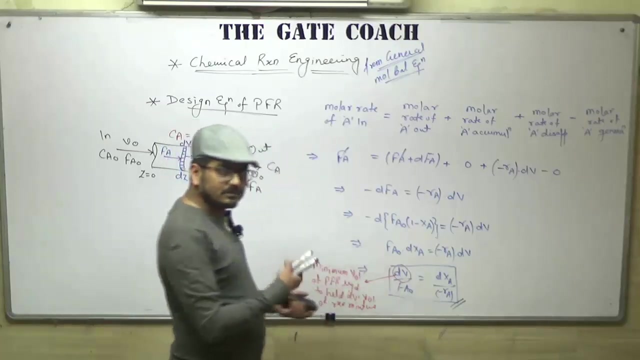 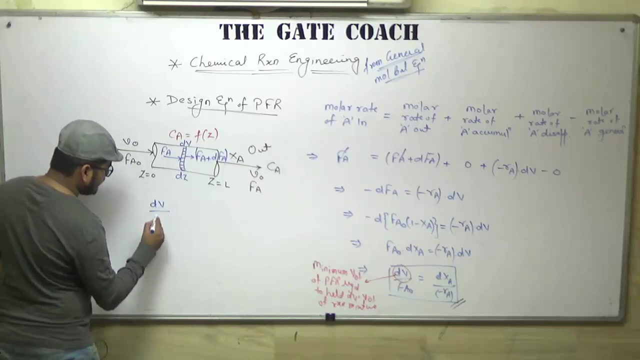 Let us do some integration and all Okay. So we have: DV over FA0 is equal to DXA over minus RA. So at DV volume of reactor at V equal to 0, the conversion of A was 0, and when we complete, 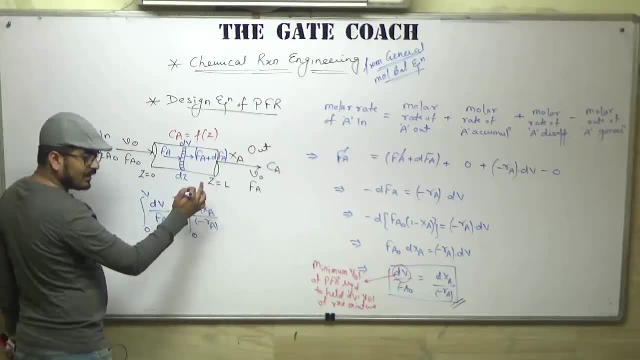 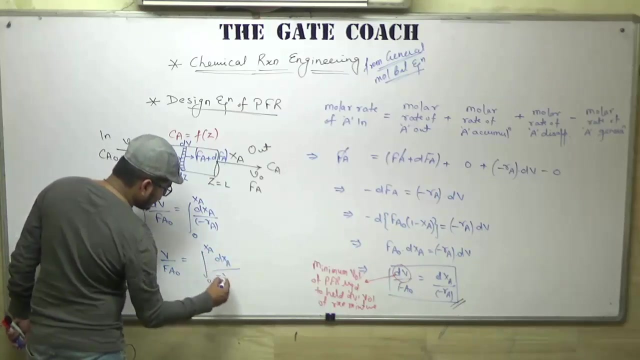 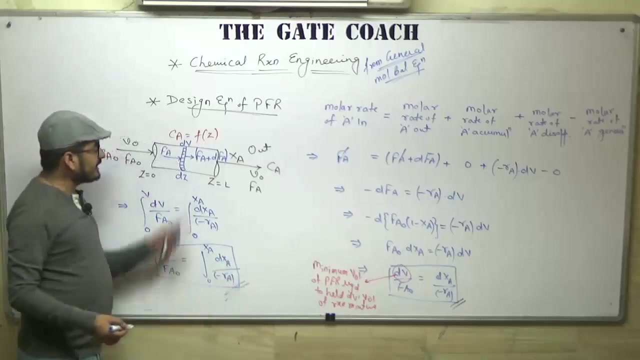 the entire volume, the entire length of the reactor V, the desired conversion will be XA. Okay, So when we integrate this, the equation will become: V over FA0 is equal to integration from 0 to XA of DXA over minus RA, and this is the design equation of ideal PFR in terms. 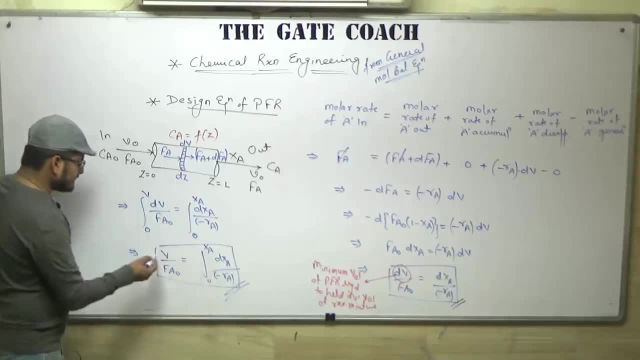 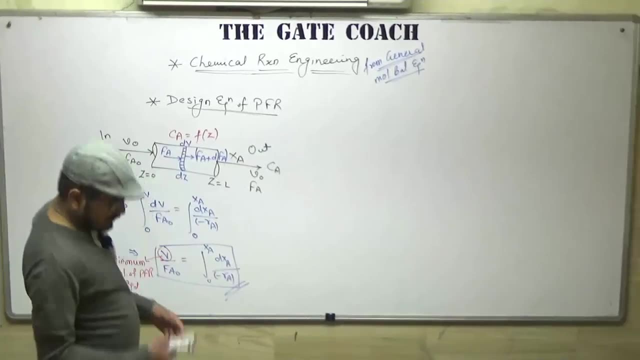 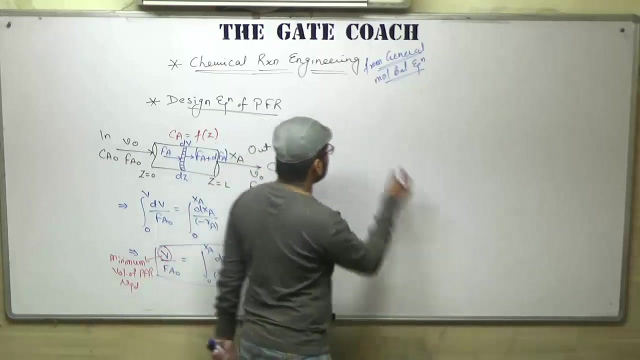 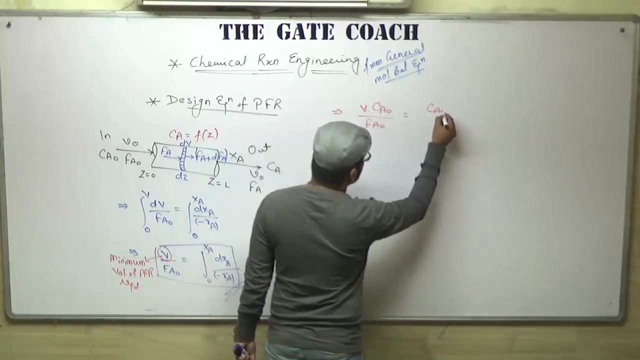 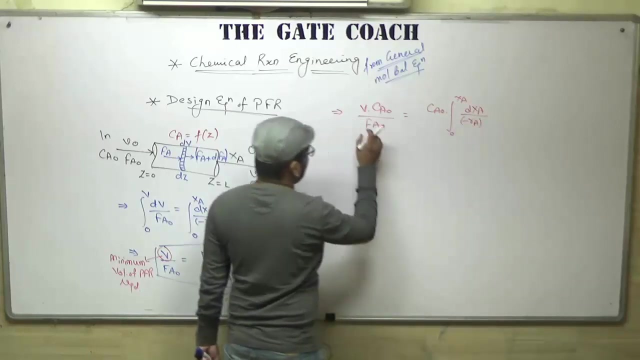 of conversion in integral form. Okay, Where this V is the minimum volume of PFR required. Okay, Now we can change this as if we multiply this equation by CA0, both side, it will become V into CA0 over FA0 is equal to CA0 into integration, from 0 to XA, of DXA over minus RA, and we know. 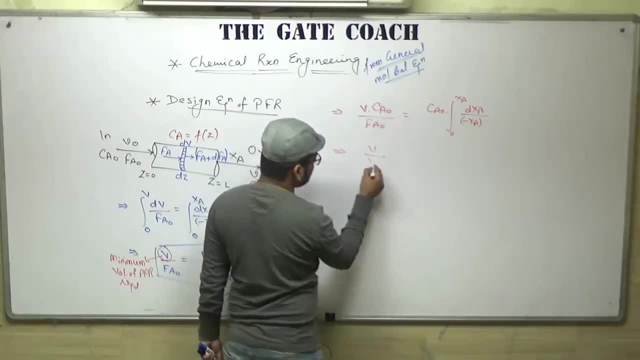 that FA0 over CA0 is like V0, the volumetric flow rate. Okay, Okay. So what is the volumetric flow rate of the reactor? What is the volumetric flow rate of the reactor? So we can write the volumetric flow rate of the reactor as TAU. 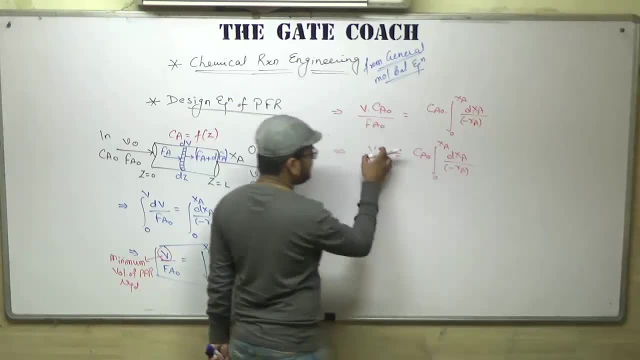 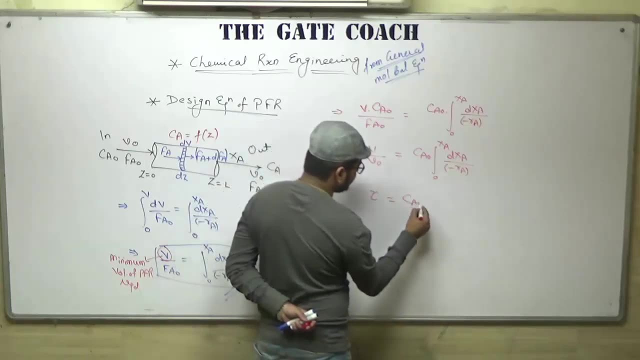 And volume of reactor divided by volumetric flow rate is what Space time? So you can write it as TAU. So ultimately we can write our design equation as: TAU over CA0, V over TA0 is equal to TAU over CA0, TAU over CA0, V over TA0. 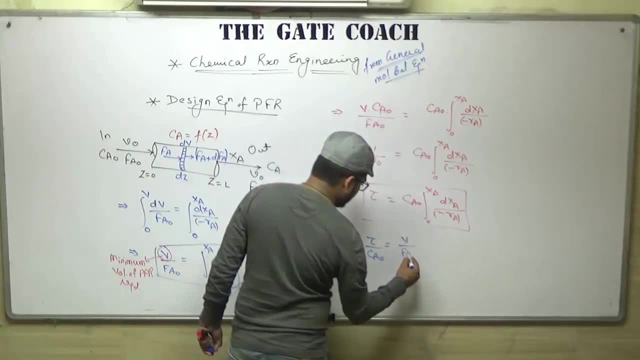 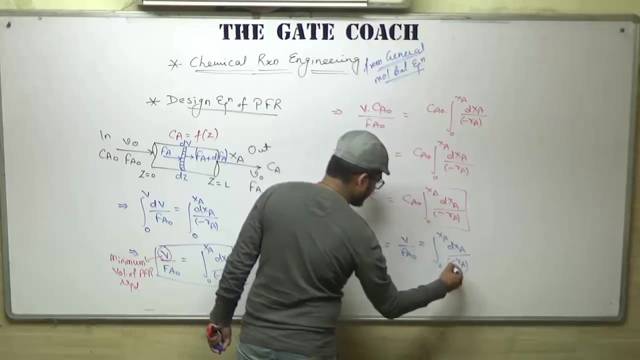 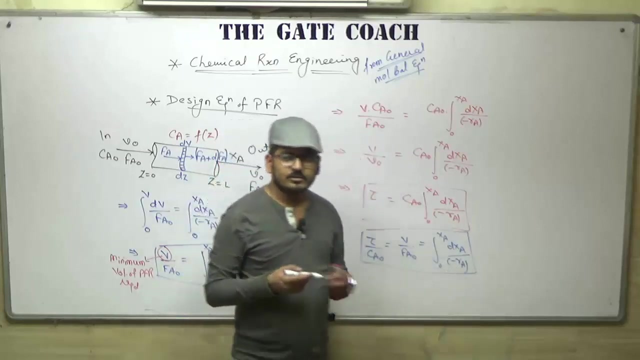 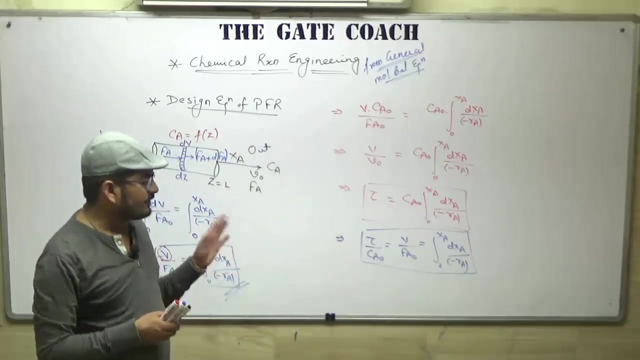 Okay, V over FA0 is equal to where, for any order of reaction, you can put the value of Ra, the rate equation, and you can solve this. This is the thing, this is the generalized form of design equation for ideal PFR, and we can write it, as we can use this equation for: 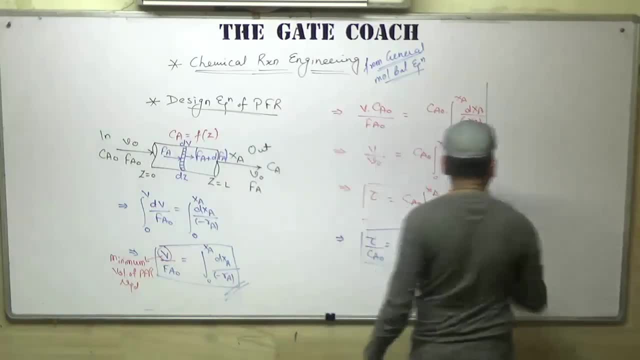 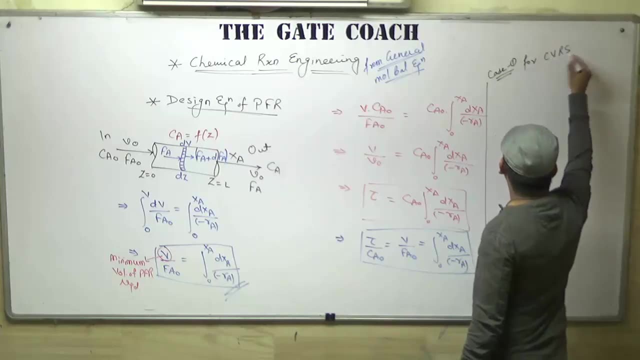 different cases as well. For example, we want to use for constant volume reaction system where volume of reaction mixture at any time, t, will be same as the initial volume of reaction mixture. So for these cases, we know that Ca is equal to Ca, n is equal to Ca p. So for these cases, we know that Ca is equal to Ca, n is equal. 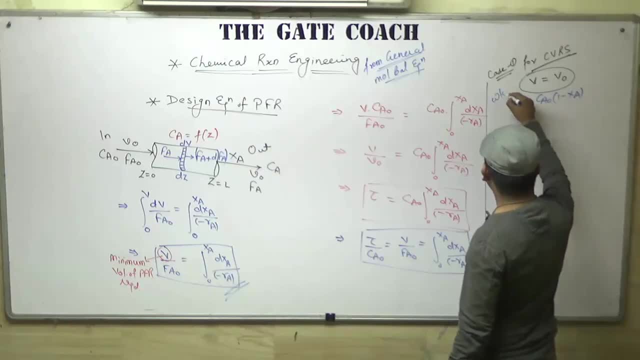 to Ca naught 1 minus Xa. We know that and we can also write it as: dCa is equal to minus Ca naught into dXa. So when you put this value in this equation you will get: tau is equal to minus. integration of dCa over minus Ra from at Xa equal to 0, Ca will be Ca naught. 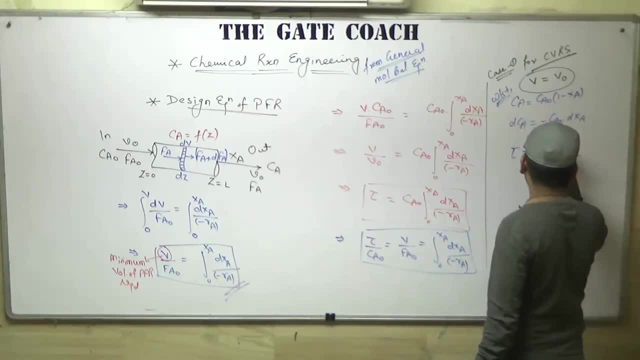 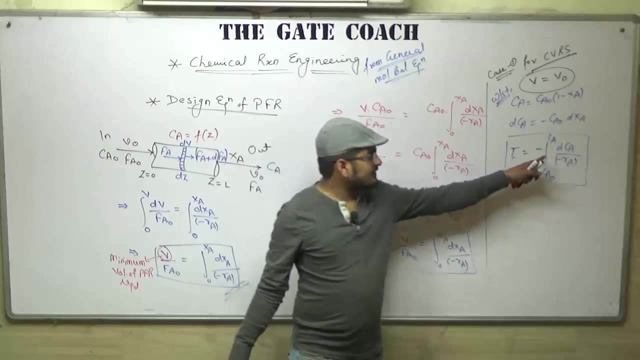 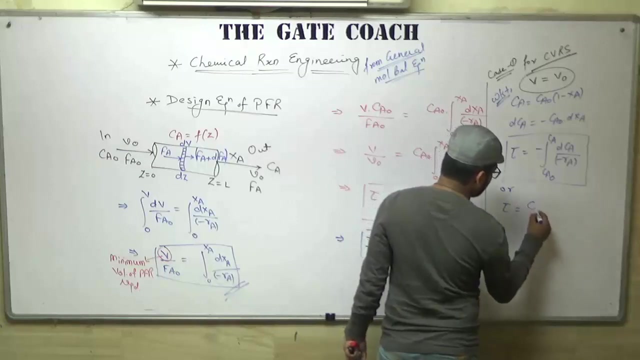 and at Xa it will be Ca. So this is the design equation of ideal PFR in terms of concentration in integral form. or we know that tau is equal to Ca, naught 0 to Xa, dXa over minus Ra in terms of conversion, This we have already derived and in these kind 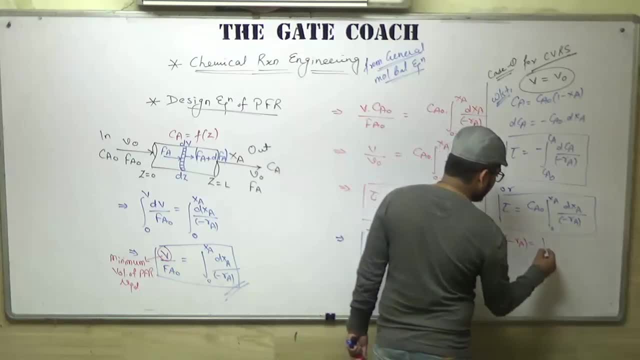 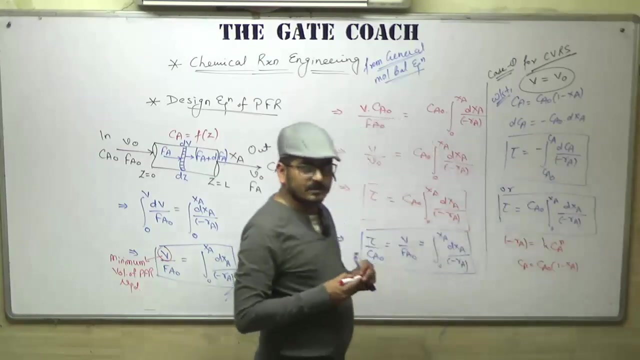 of cases. we know that we can write Ra with the help of power law, as K, Ca, power n, For example, if one reactant is here and we can write Ca as Ca naught 1 minus Xa. So put this value n, this equation and solve Simple. 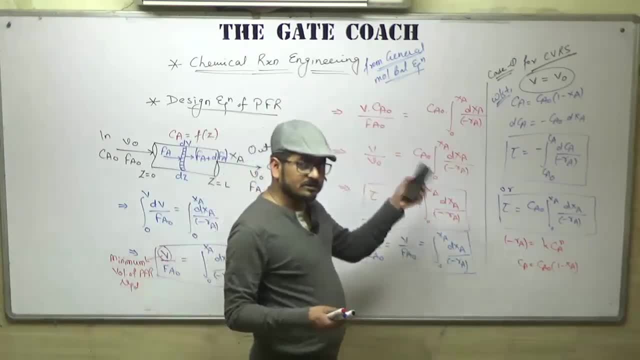 When you draw these design equations, also known as performance equation, over a curve, it will be like: What is the result? 5, 0.8,. let us condition that per unit weight, or equal to 2.. embora by 3.4,lo. here we have cut speaker vitamin A 0.2 by xa. How many repetitions there. 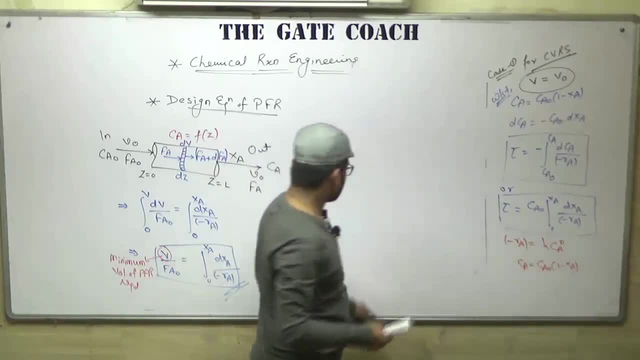 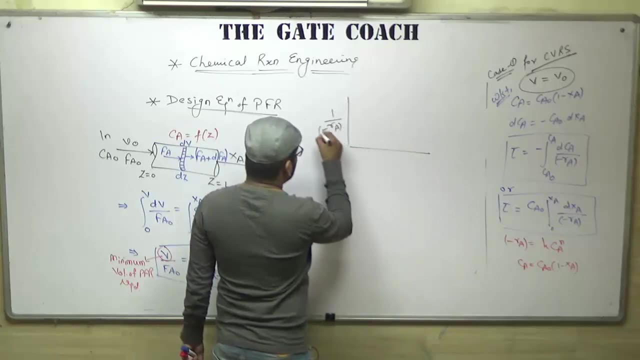 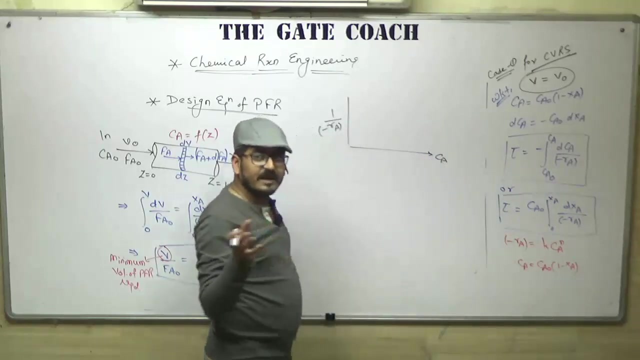 are. Let us condition that every set of reacting to each other surface is equal to 0 in Cav, around Q1,34 per unit. When we draw the curve between 1 over Ra versus Ca, we know that in the reaction mixture the initial concentration is Ca naught and which is the higher value of Ca and the final concentration. 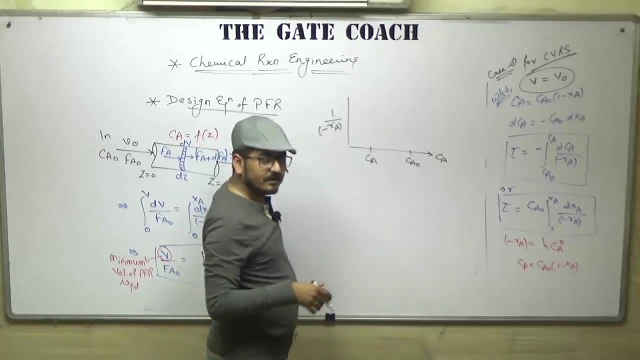 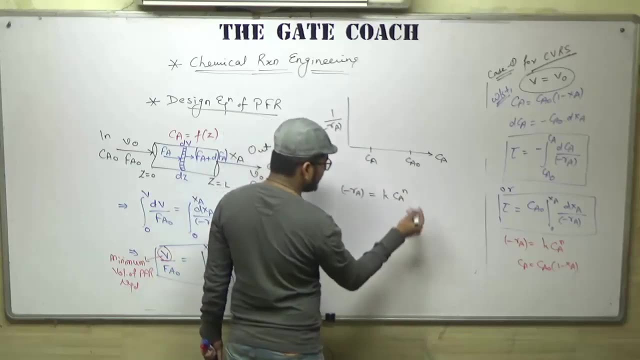 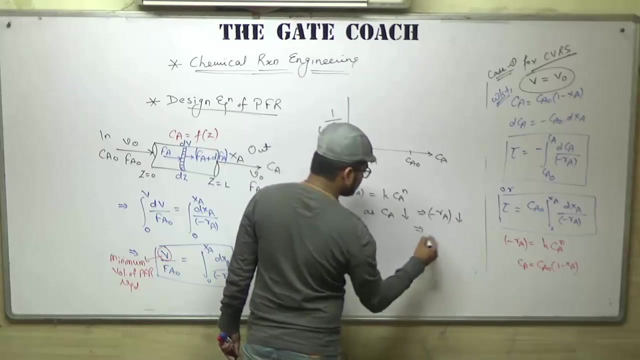 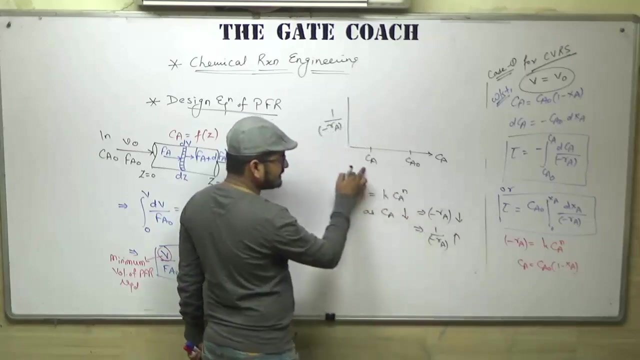 is Ca, which is the lower value of Ca. So the curve. we know that Ra is equal to K, Ca power, something. So as Ca decreases, Ra will decrease. Thus the 1 over of minus Ra will increase. So in this direction, as we are decreasing, this will increase. This is Ca. 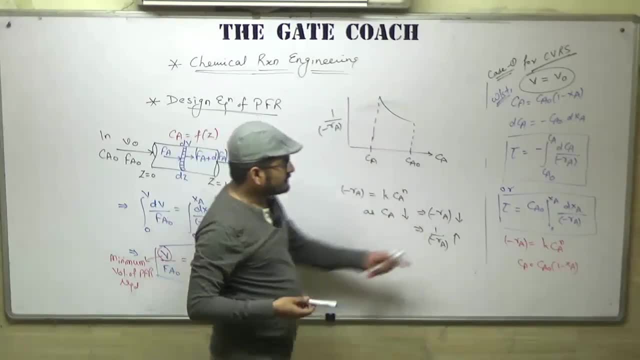 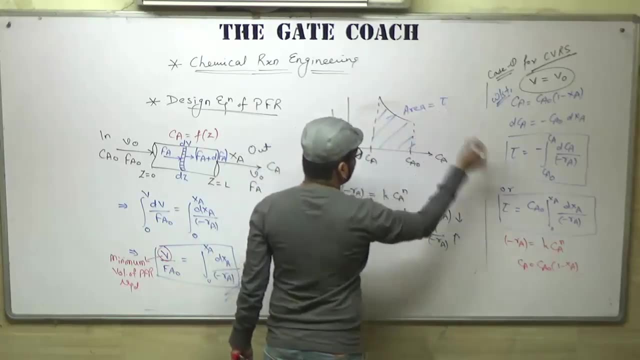 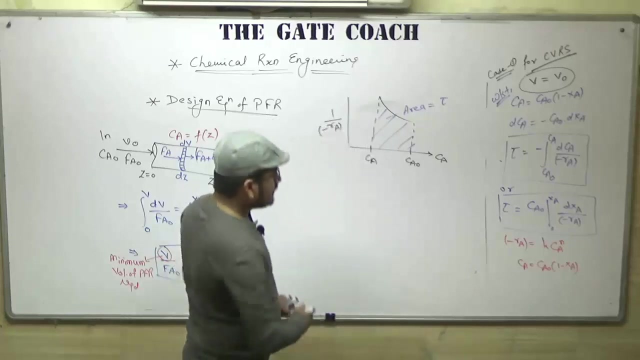 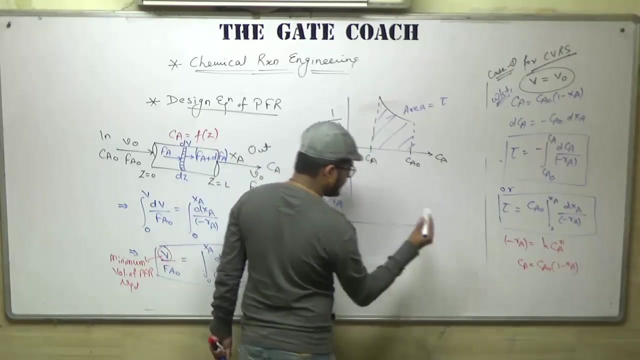 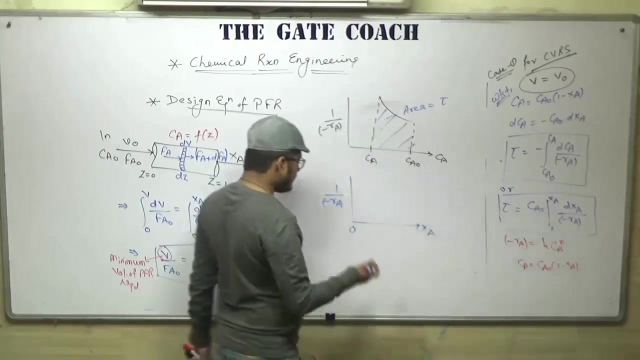 this is Ca naught and this is the performance curve And because of the integration sign, we will consider only area under the curve, which will be equal to Tau. We can see that. And for second case, if we draw the performance curve between 1 over Ra versus Xa, as we can see, from 0 to Xa, we know it will be equal to. 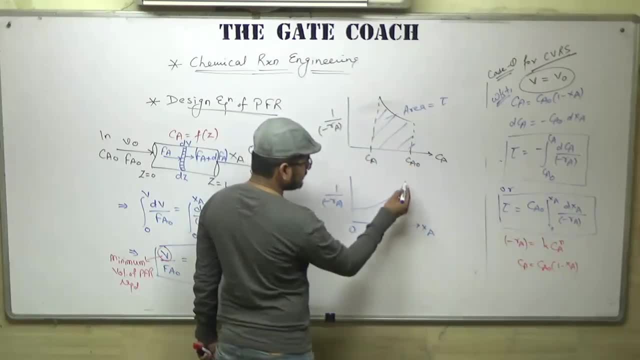 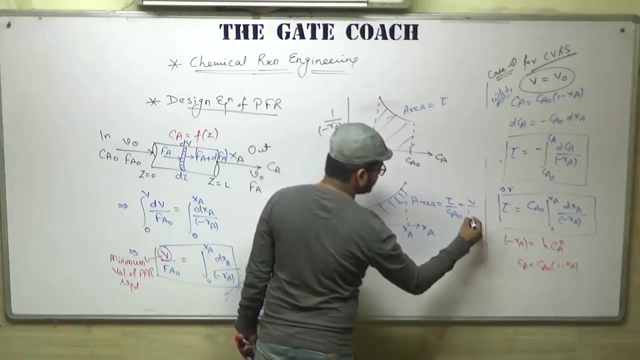 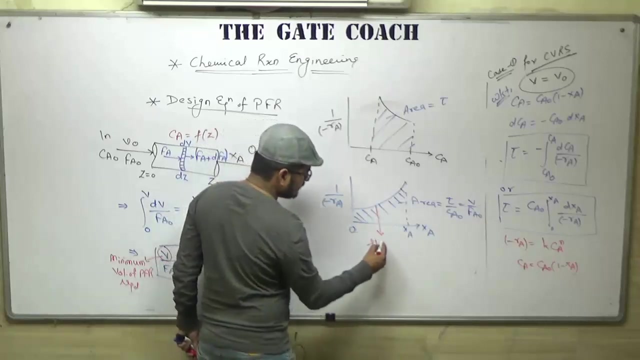 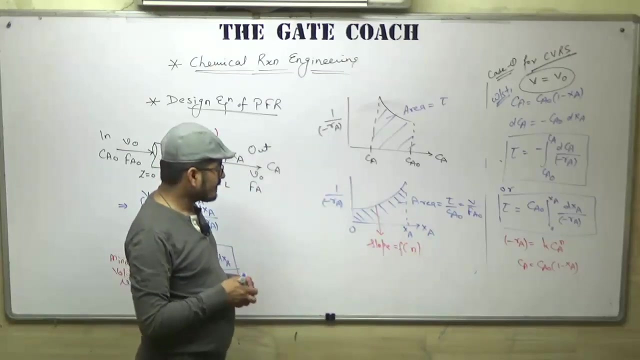 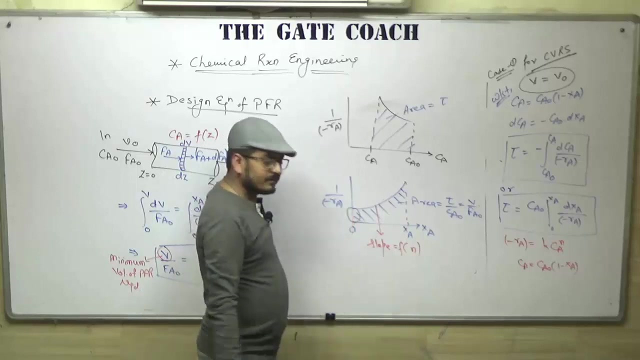 Tau by Ca naught, or you can also write it as V by Fa naught. And the thing, the slope of this curve depends on the order of reaction. And now my question is why this curve is not starting from 0? Why it is starting from here. 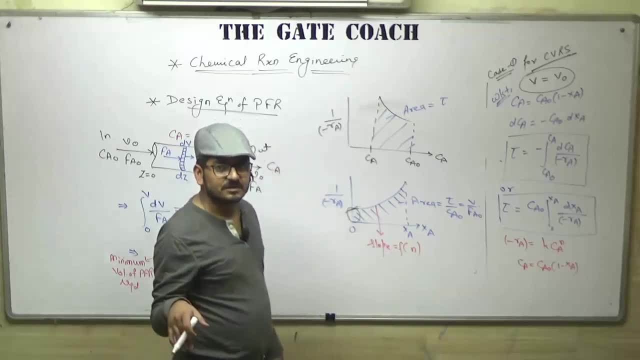 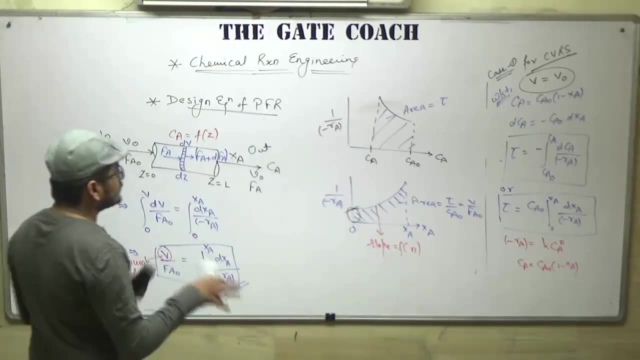 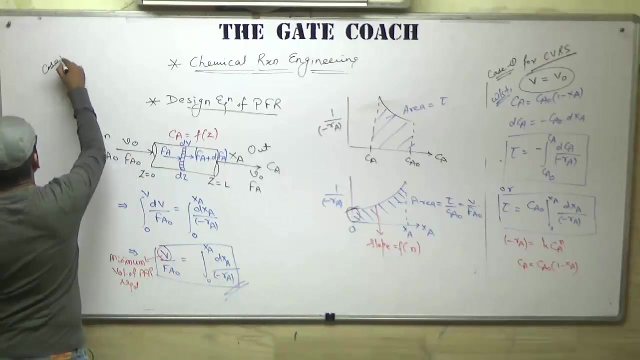 You know that, It is very well, Then answer in the comment section. If you do not know, then you can ask. So this is something about the designing of PFR. Let us also talk about the second case, That is, for variable volume reaction system, where we know that the volume of reaction